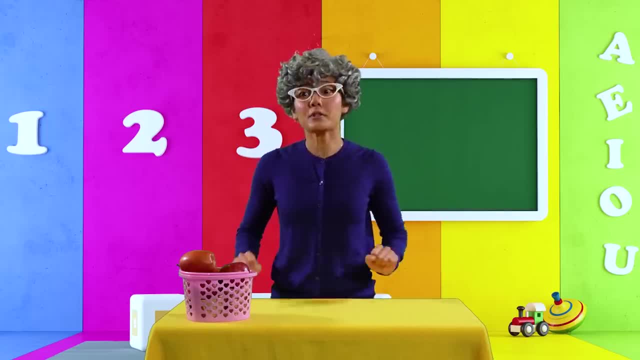 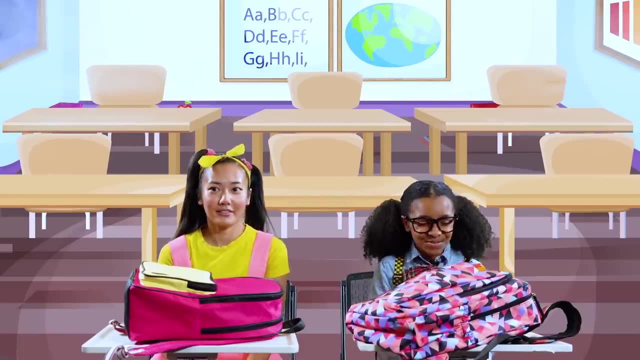 I can't wait to see how silly your hats are. Who's going to start first? Oh, me, me, me, me me, I go first. I go first, since I always follow the teacher's rules. My hat was made exactly how you said, Miss Blue. 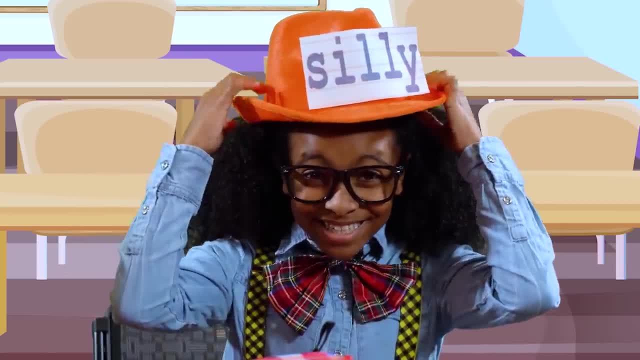 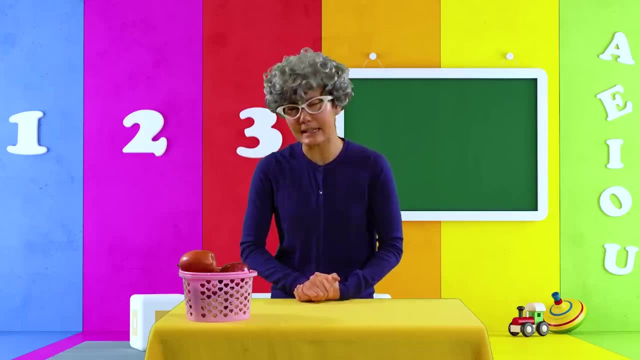 See, here's the word silly, and I can wear it on my head. It's a silly hat, Just like what you asked for, Miss Blue, right? Well, that definitely is a silly hat, but I was expecting something a little more silly. 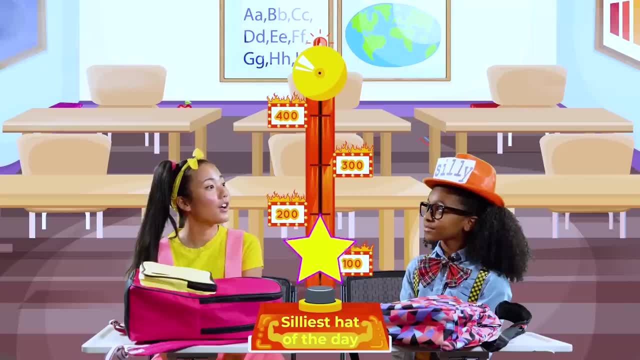 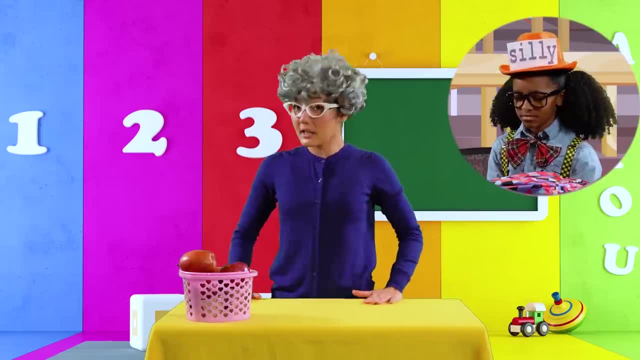 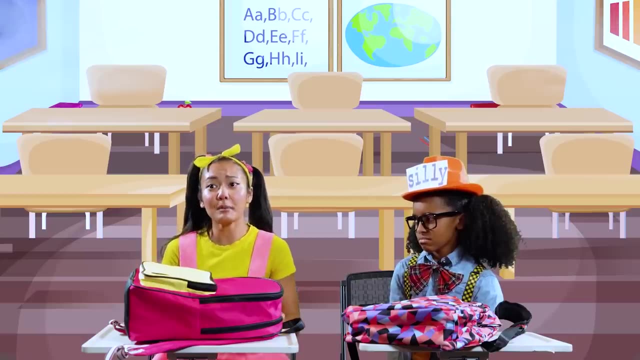 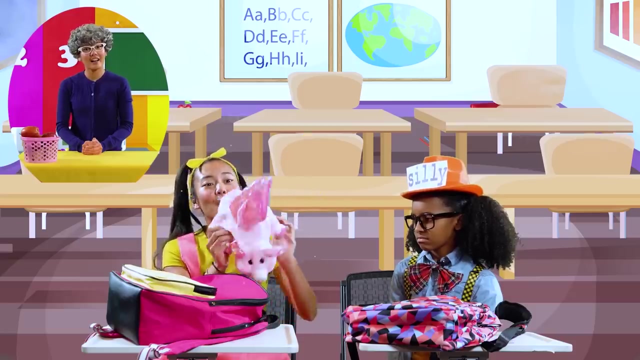 Let's see what grade the silly meter gives your hat. Well done, Alex. The silly meter gives your hat two points. Now let's see what Ellie's hat is like. Well, my hat is a little bit different from Alex's. I made it- and it's one of my favorite animals- a pig with wings. 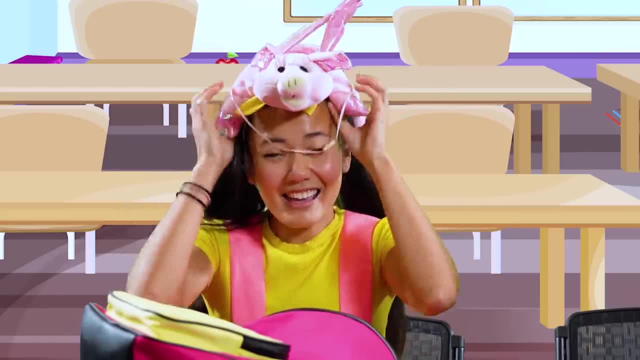 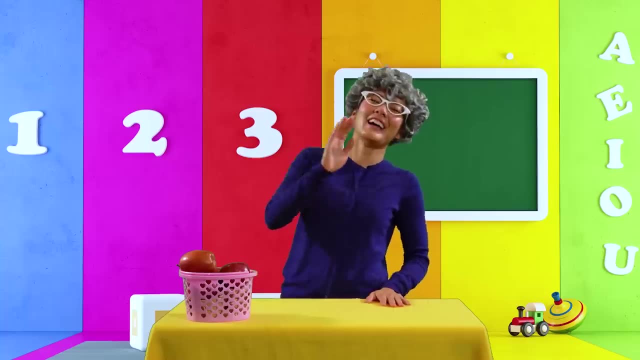 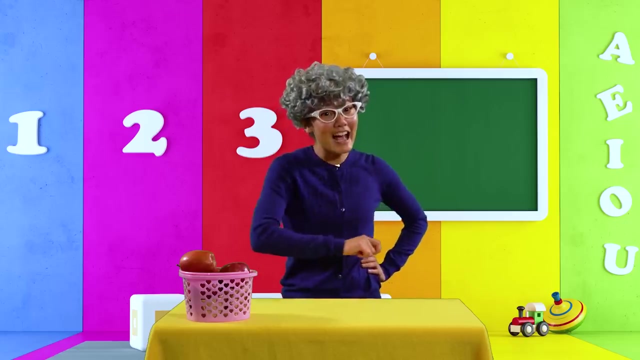 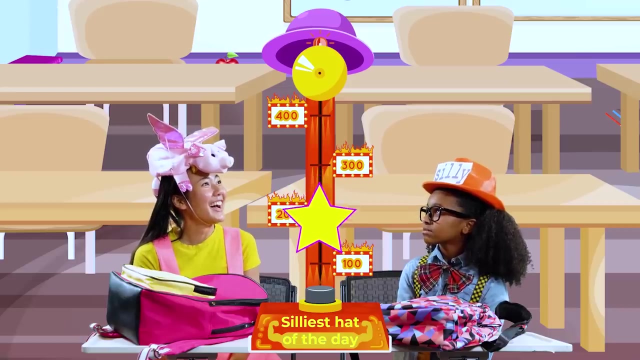 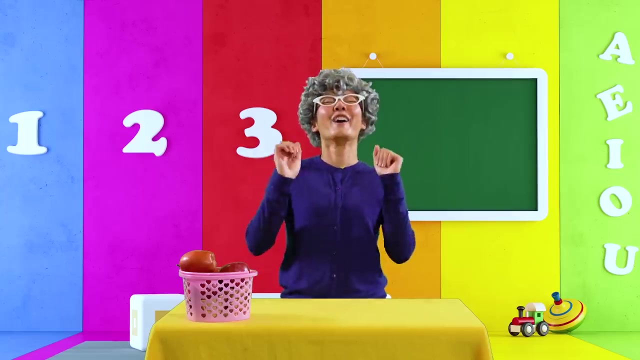 You can even make the wings move like this. A flying pig hat. Now that is a silly hat. I can't wait to see what the silly meter says about your hat. One, two, three, four, five, Wow, Those are five silly points from you, Ellie. 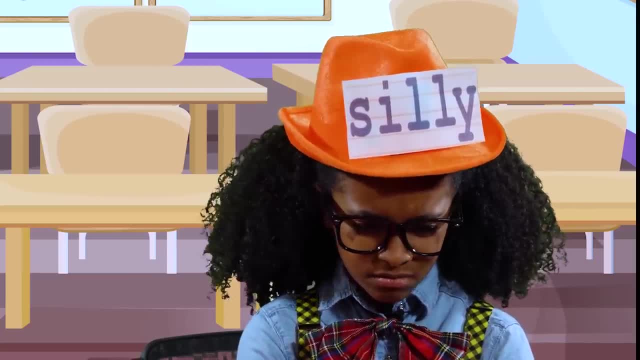 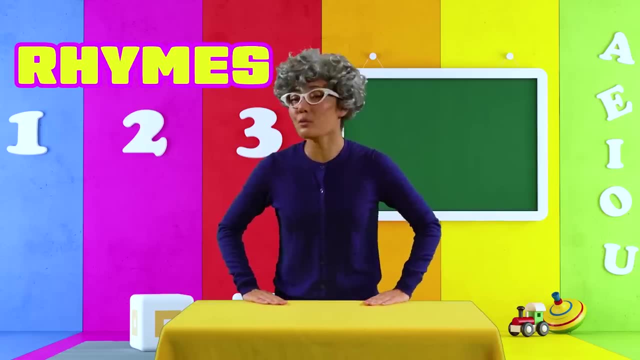 I think your hat was so silly it broke the silly meter. It's not even silly or funny. My hat was silly and funny Rhymes. Rhymes are when two words have the same sounds at the end, For example king. 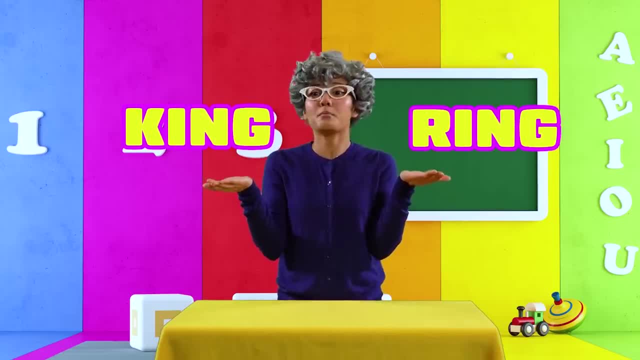 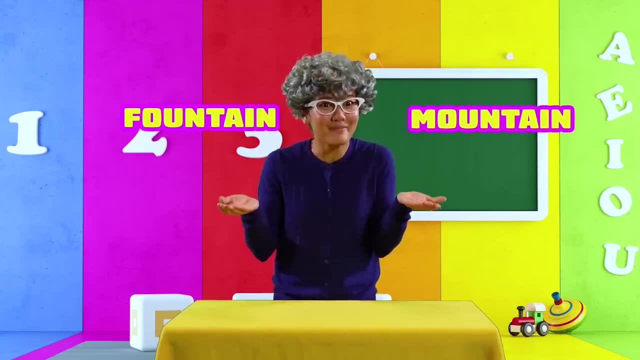 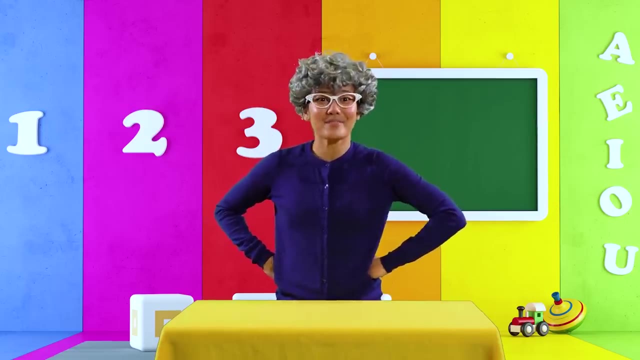 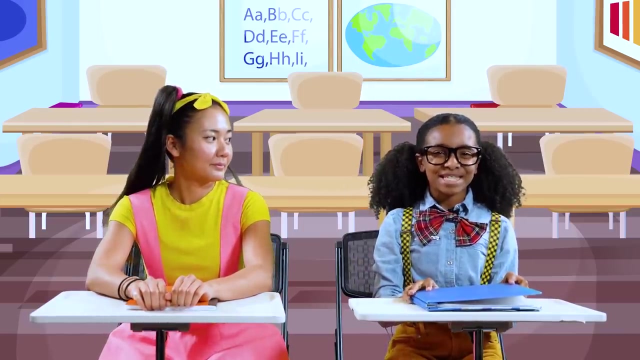 rhymes with ring. The king bought a ring. Now here's one that's a little harder. Fountain rhymes with mountain. There's a fountain on top of the mountain. Now you have to tell me a short poem that rhymes. Who will start? I will. This poem is called Miss Blue Roses. 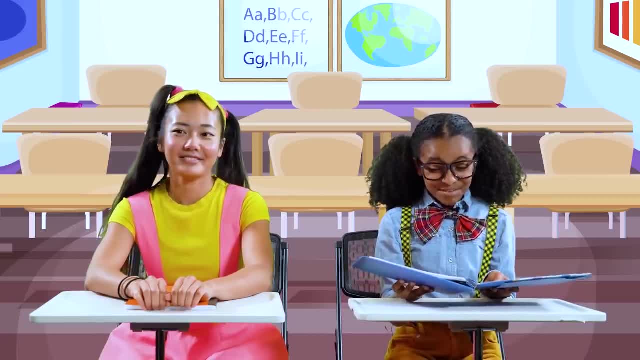 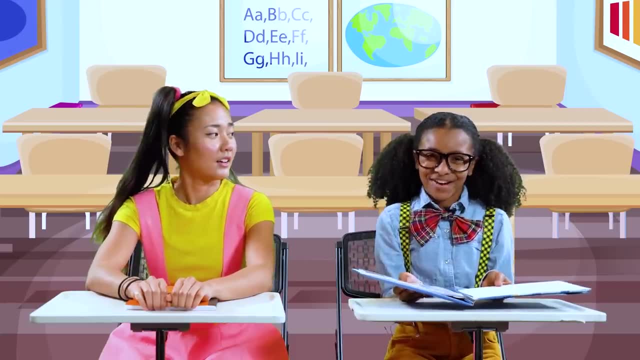 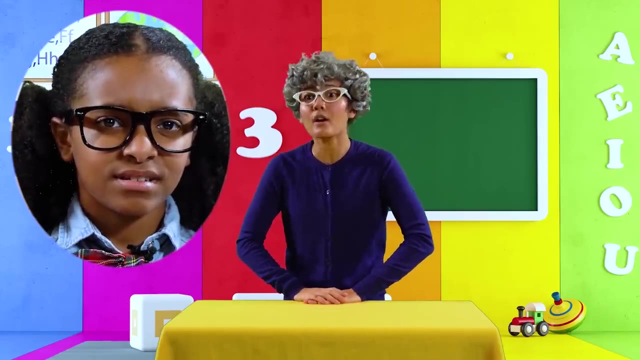 are red, Violets are blue And, speaking of blue, Miss Blue is the smartest teacher in the whole wide world And she is my hero. The end, Well, that was very nice, Alex, But your poem didn't exactly rhyme. Remember, rhymes are when two words have the same sound. 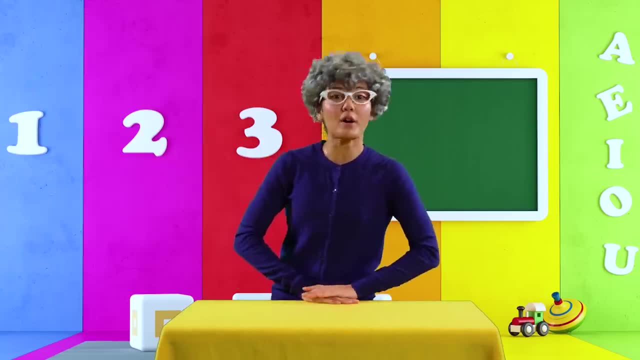 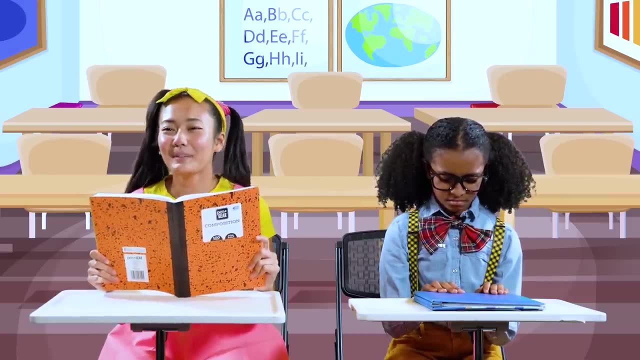 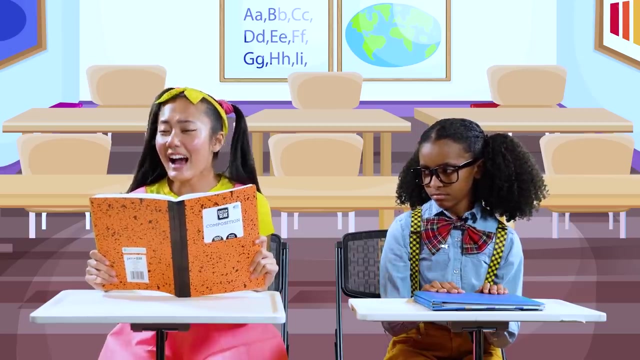 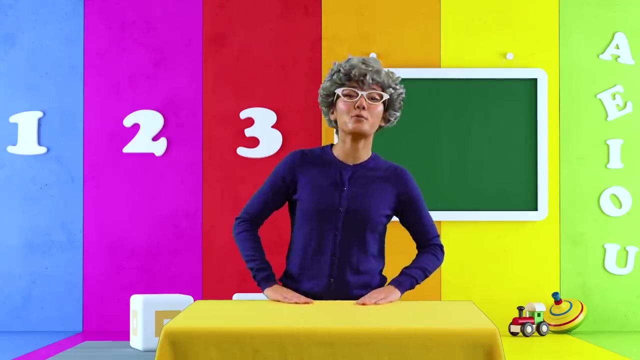 at the end. Ellie, what about your poem? My name is Ellie and I like to eat cheese. I always mind my manners, so I always say please. I say please, can I have some cheese? Not, please, can I have some peas? I don't like peas, I only like cheese. Oh, Ellie, what? 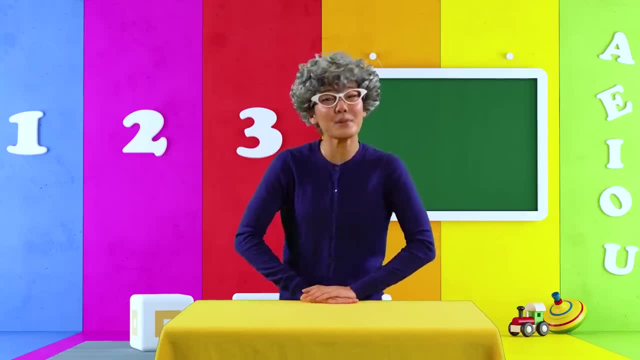 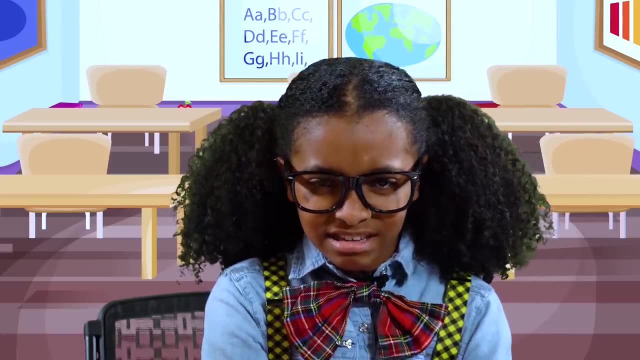 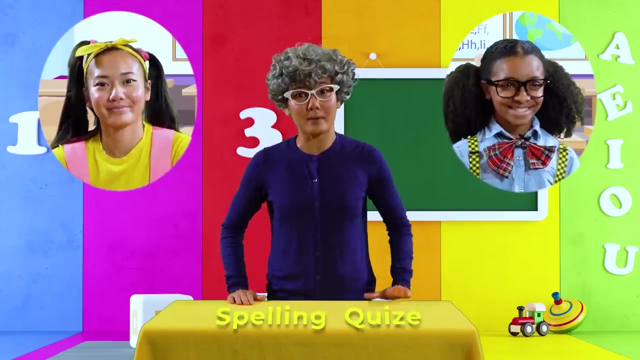 a wonderful poem. Not only did it rhyme, it was also super silly. A plus for you, Ellie. Well done. Not again. I can't let Ellie keep doing better than me in class. Now that we've learned all about rhyming, it's time for our big spelling quiz. First question: What letter? 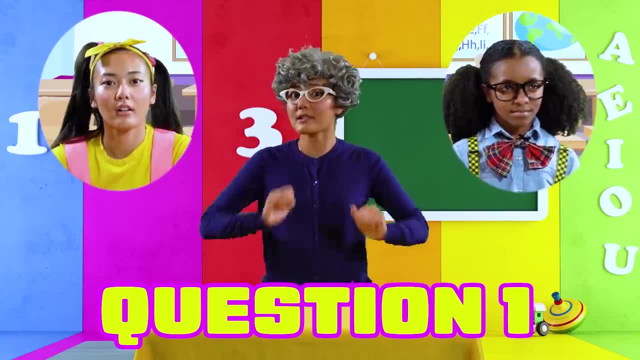 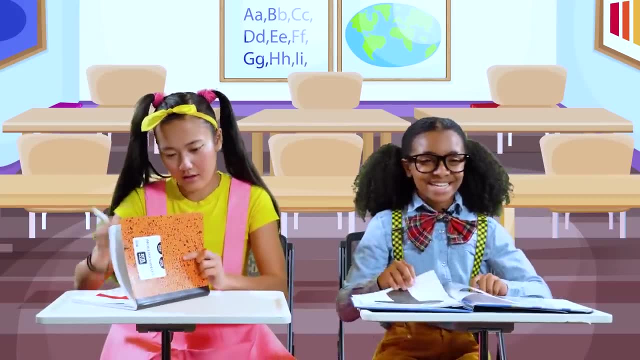 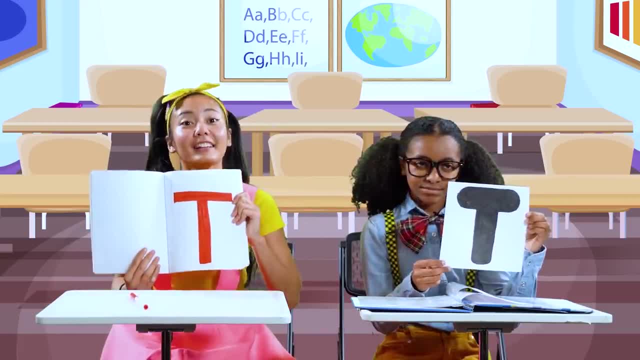 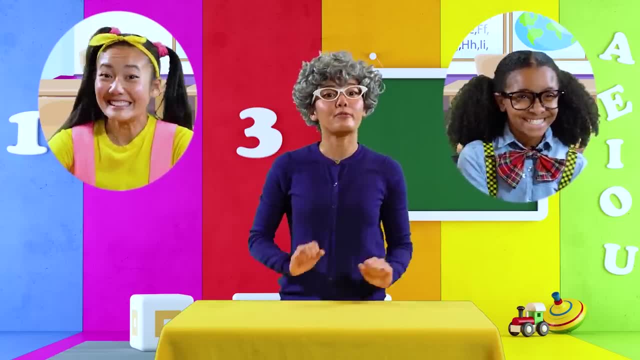 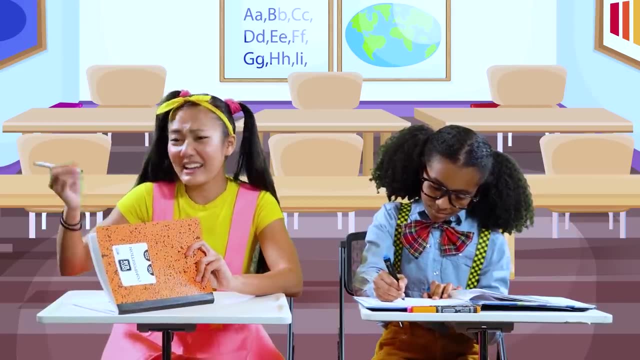 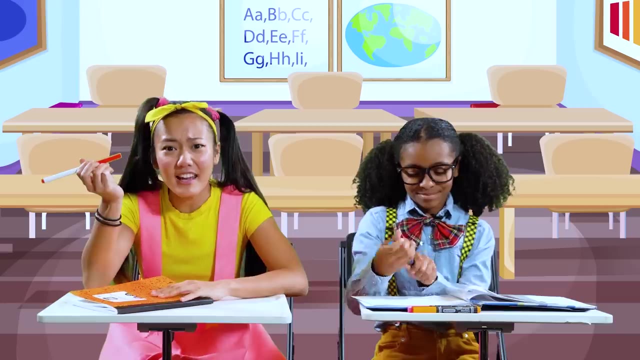 down. question two: I want you to use your favorite marker and write the word school. Uh-oh, Wait a second. My marker's all dried up and it was the only marker I brought today. Oh no, Hey, Alex. 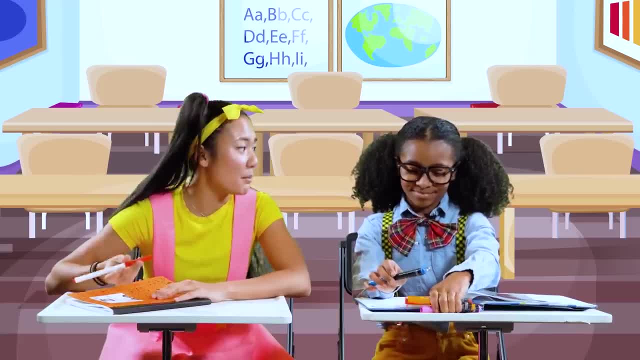 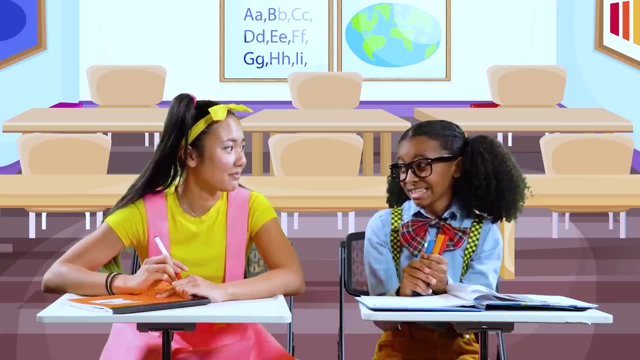 Do you mind if I borrow one of your markers? Mine just dried up. Sorry, Ellie Sparkles, but I never let anyone borrow my markers. That's why you're supposed to bring extra markers for the test. But I promise I'll give it back to you after the test. Oh Okay, everyone. 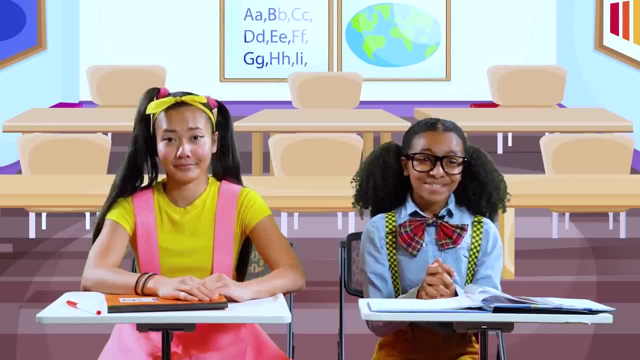 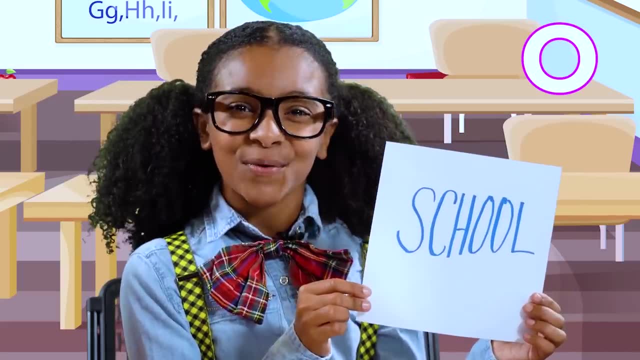 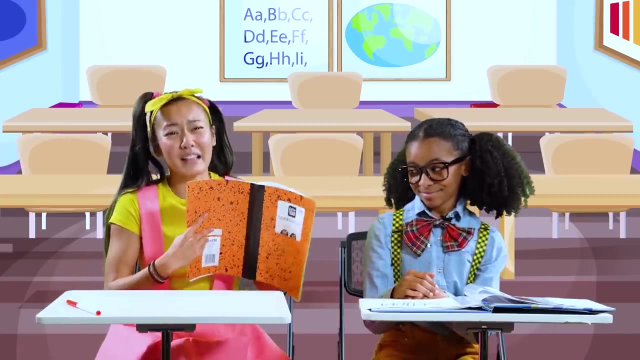 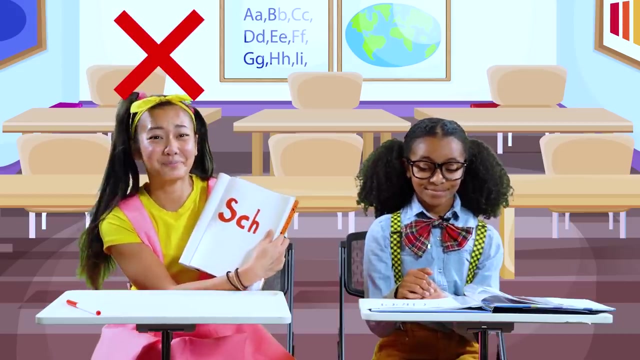 Time's up. Let's see your answers. Miss Blue, this was a hard one, but I know exactly how to spell it: C-S-C-H-O-O-L School. Um, Miss Blue, my marker dried up in the middle of it after S-C-H, So that's when. 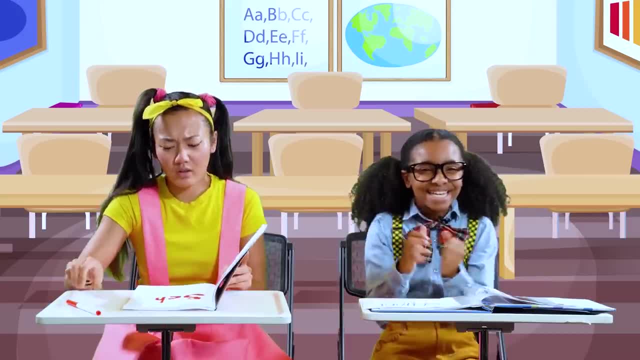 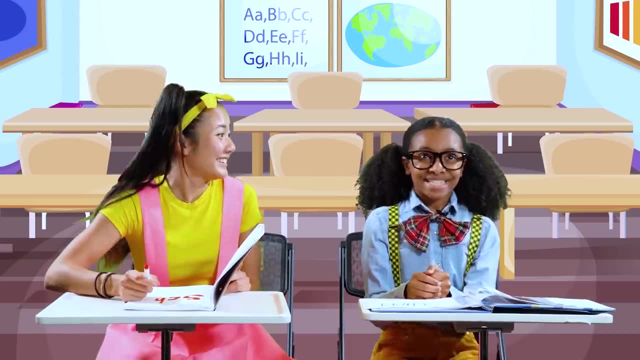 I wrote: Yes, yes, yes, I got them all right. That's why I'm the best student in your class, Miss Blue. Oh, it's time for lunch. What a wonderful morning it was. Wow, What's going on? 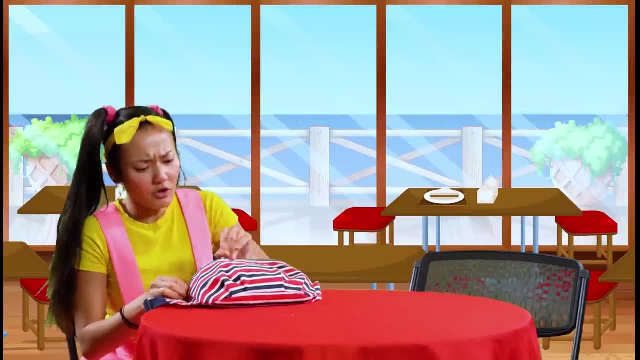 Oh no, You didn't bring the markers. Oh okay, Okayrine, What did you bring My number? We sure did a lot of things in class today, and now I'm super hungry. Lucky for me, I have my favorite lunch. 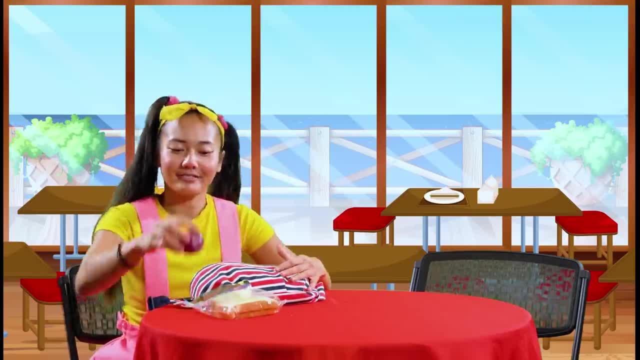 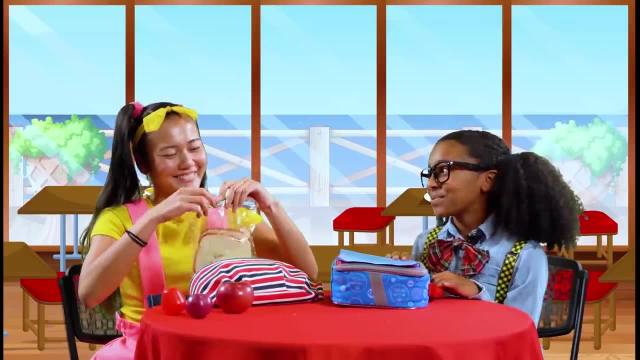 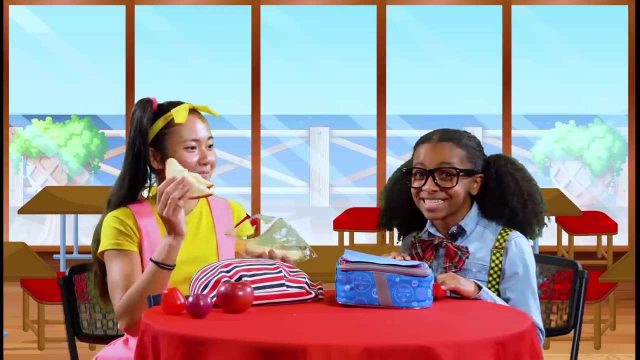 Peanut butter and jelly sandwich and some fruit. Oh, hello, Lee Sparkles. That was a great spelling test, wasn't it? Yes, What do you have for lunch? A peanut butter and jelly sandwich. Mm-hmm Well, I have something much, much better. 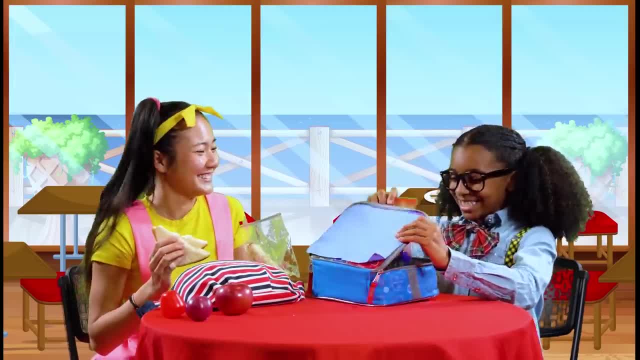 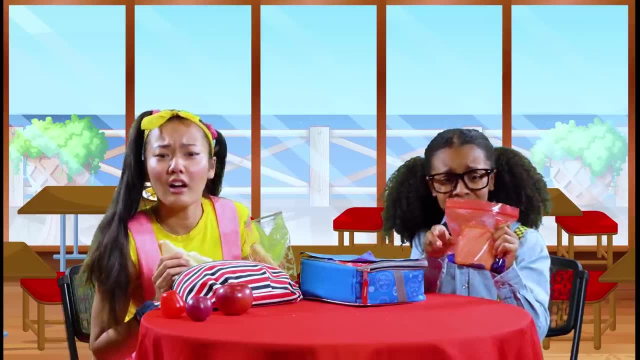 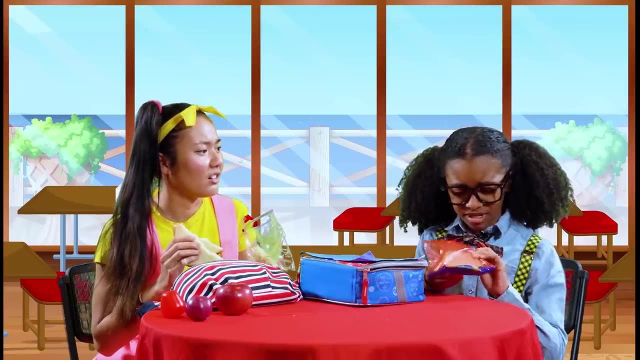 A blueberry ice cream sandwich. See, I told you my lunch was way better than, Oh no, my sandwich. It's. it's melted. I must've forgot to put the ice cream in the freezer. Oh, it's okay, Alex. 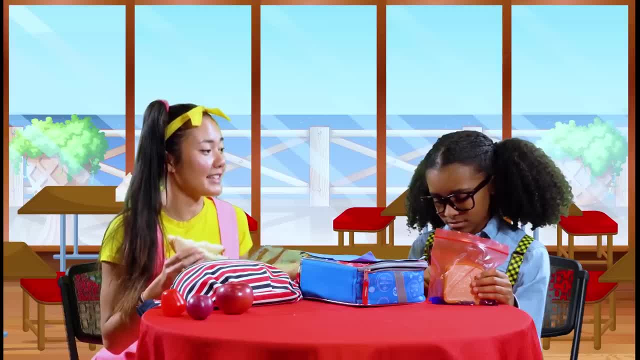 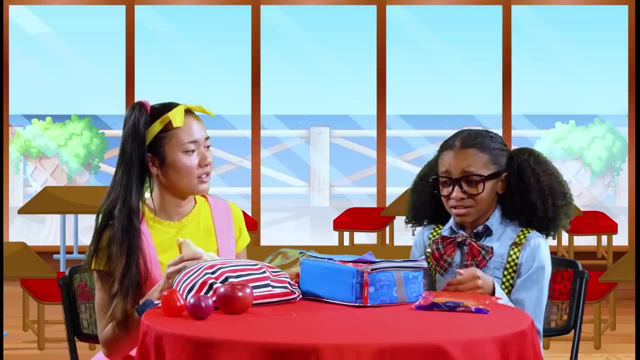 You can share my lunch with me. I have another half of peanut butter and jelly sandwich, Are you okay? No, I'm not okay. Miss Blue likes you more than me because you do everything right. Your silly hat was way sillier than mine. 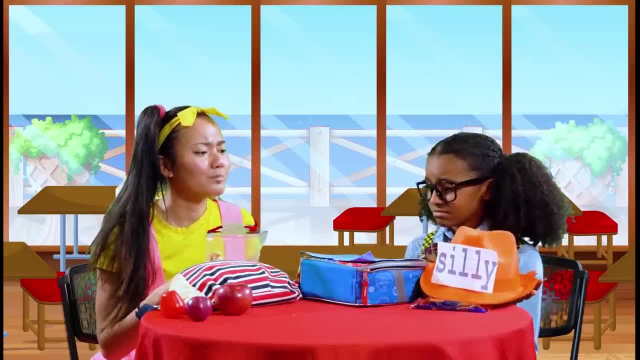 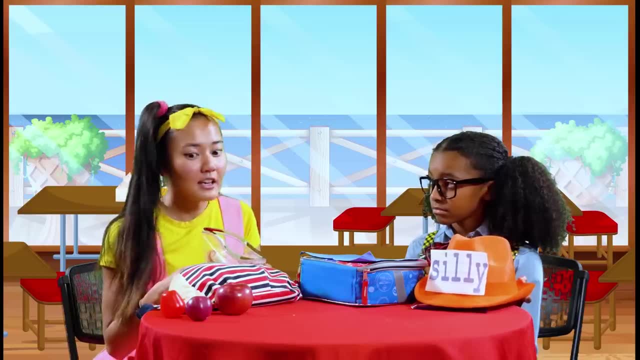 and your poem actually rhymed: Mm. you're upset about your hat. Well, I have a great idea. I'm really good at making things silly and I have all these fruit. Maybe we can use my fruit to make your hat super silly. 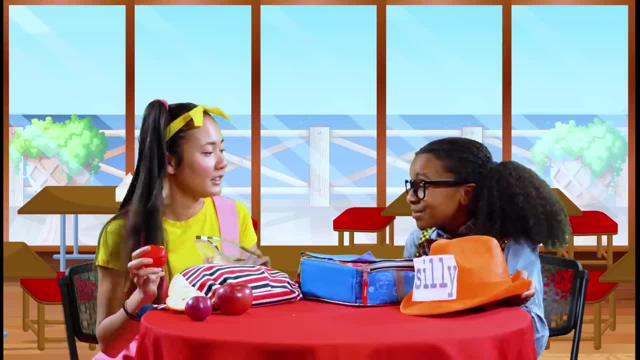 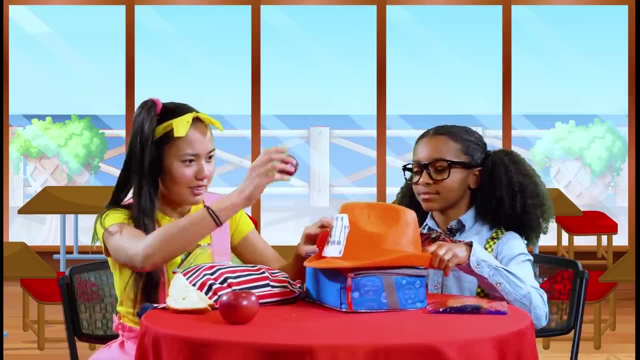 How does that sound? Great idea. Ellie Sparkles, Do you think you could teach me how to rhyme too, Of course? Well, let's get this hat all silly'd up. The name of this poem is called My Friend Ellie. 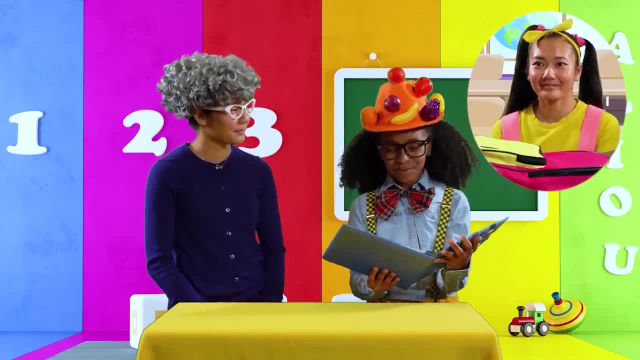 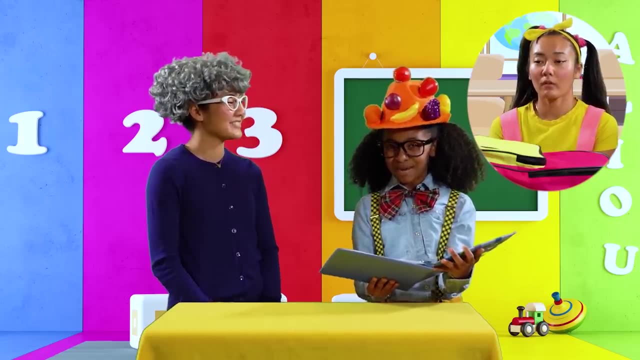 I have an awesome friend named Ellie. At lunch we shared peanut butter and jelly. When I need help in school, I know a friend. that's cool. My friend's name rhymes with belly. It's Ellie. Bravo, bravo, Alex. 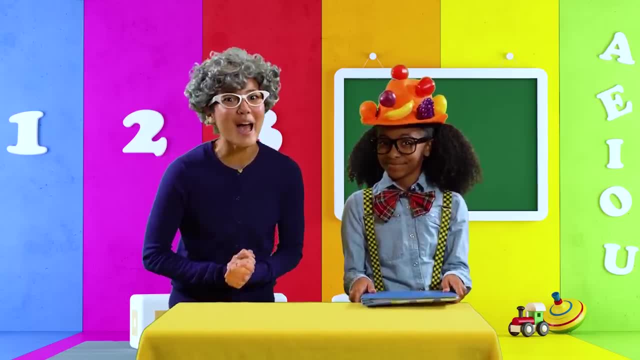 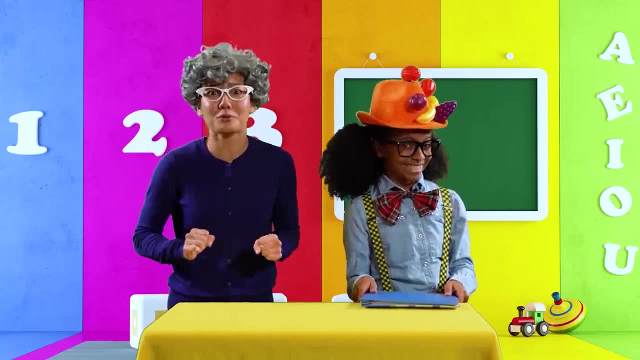 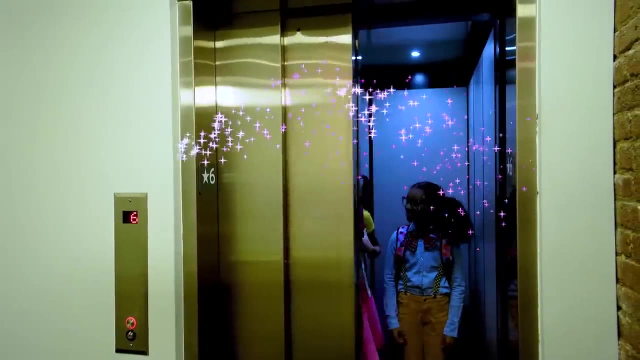 What a wonderful poem with wonderful rhymes. And this hat, This wonderful hat. It's covered in all sorts of fruits that I love. It's so silly. Oh, my goodness, just look at it. A pluses for everyone. Ellie, are you ready for my favorite class of the day? 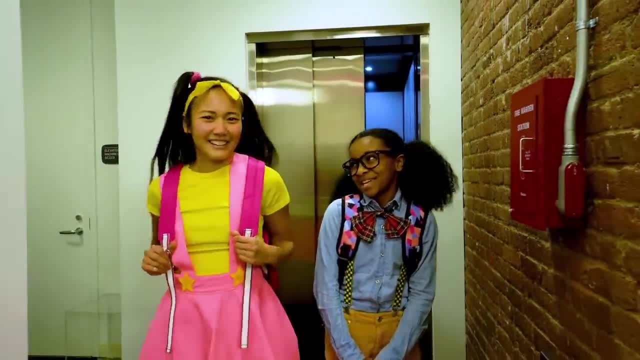 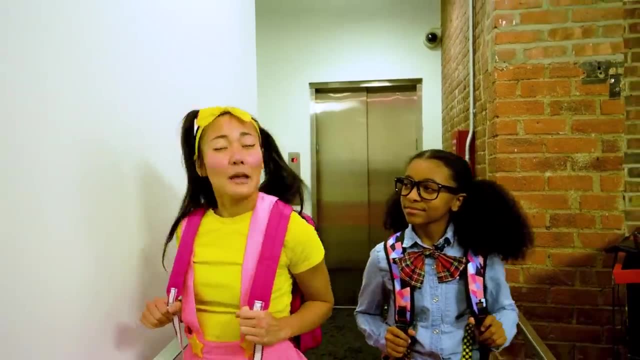 with the best teacher ever. I always get everything right in this class. I'm the number one smartest student. You are a pretty great student, Alex, And this teacher is definitely a little weird, but he's really cool. I like him a lot. 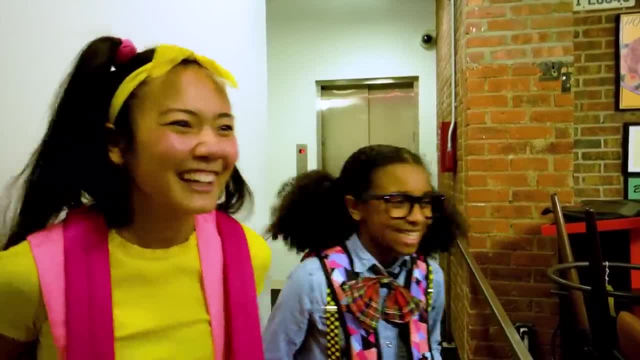 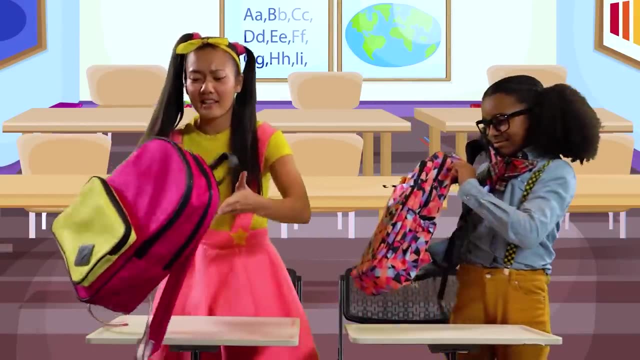 Oh, there's our classroom over there. Let's sit together today. Let's go. Oh man, I'm always worried about this class. I always think that I'm giving the right answers, but the answers never seem to be right enough. 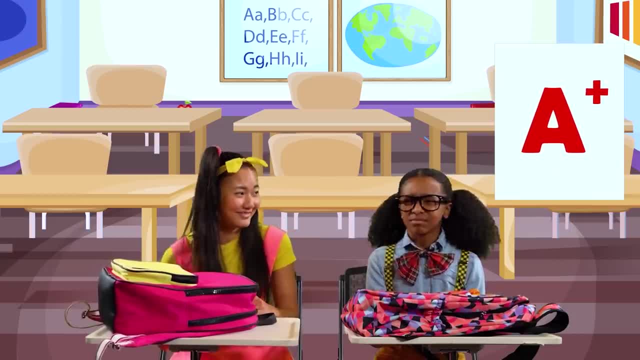 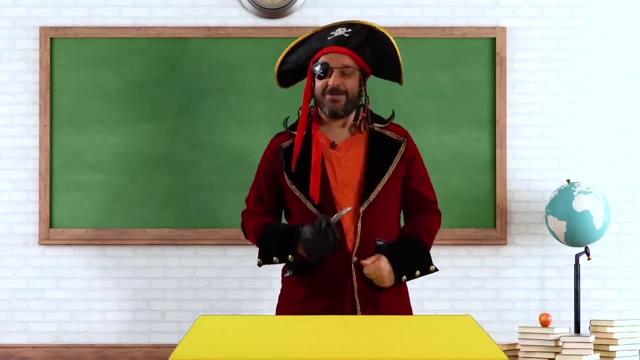 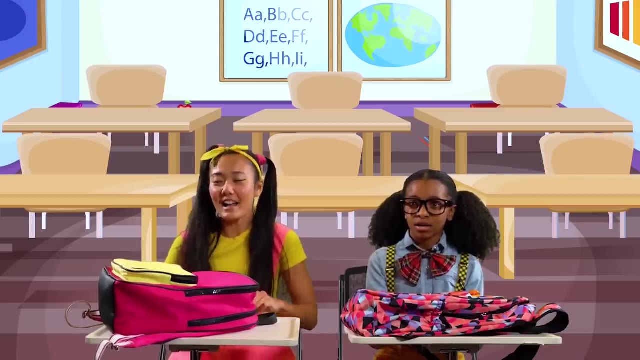 I never have that problem, Ellie, I'm always right. Hey, where's the teacher? Hello class, Are you ready for me? Pirate lesson Today is going to be extra piratey, Awesome. Oh, Mr Pirate, I have something for you. 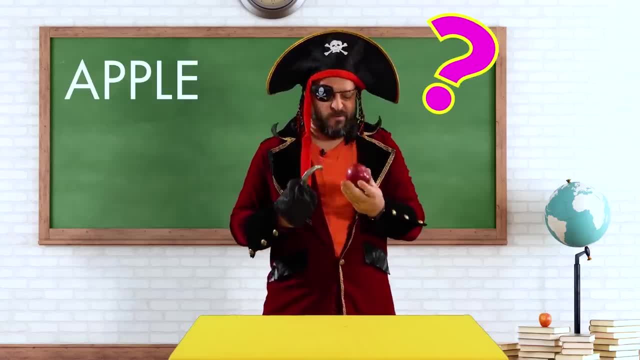 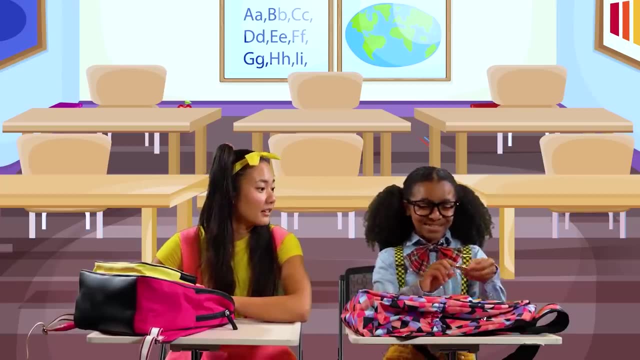 An apple. What's a pirate supposed to do with an apple? It's not very shiny, but it'll do. Mr Pirate, look at what I have for you, For me: A gold coin. Wowie, zowie, Wowie zowie. 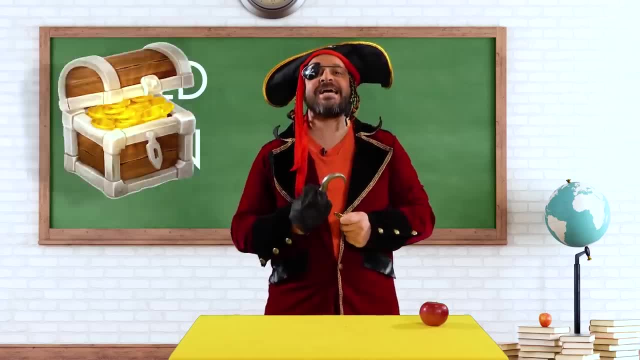 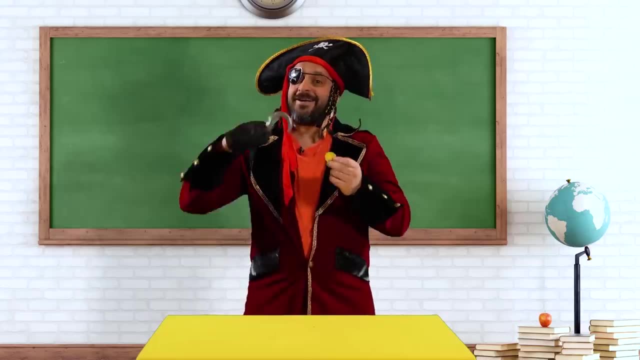 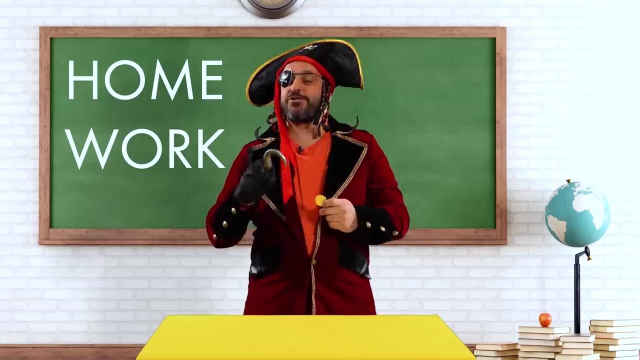 It's so sparkly and shiny, just like I like me pirate gold. You're off to a great start, Alex. Cool, Now that I have me gold coins, it's time to check your homework. Last night, I asked you to draw something super colorful. 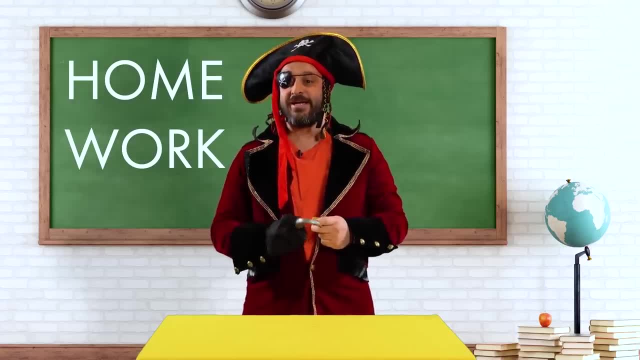 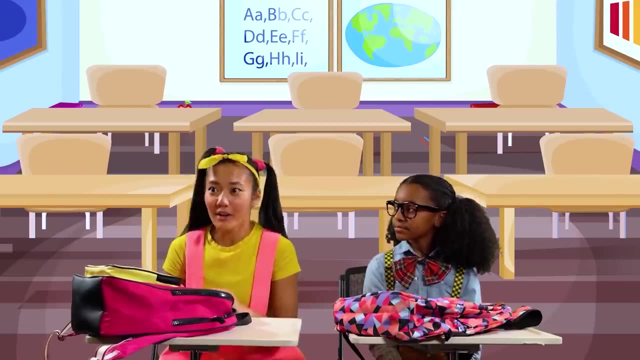 and extra piratey. So let's see what you have for me. Ellie Sparkles, you go first. Thank you, Mr Pirate. Now I love coloring with all the colorful markers, so I drew something that was super colorful as well. 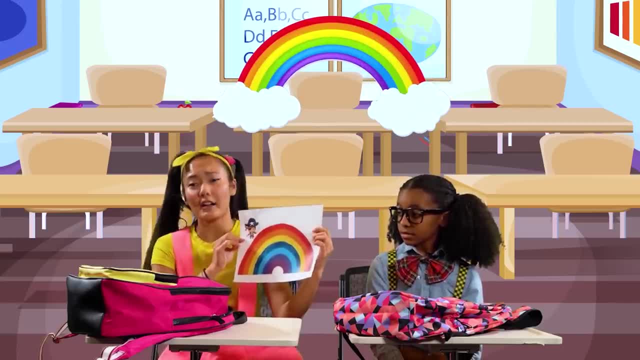 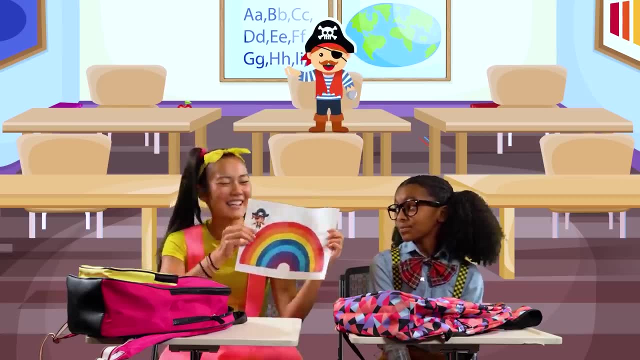 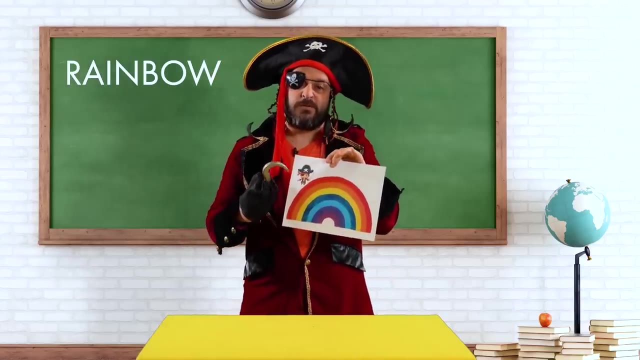 It's a rainbow. Look, it has all my favorite colors on it: Red, yellow, blue, and I even had time to draw a picture of you, Mr Pirate. Ah, a rainbow. That doesn't seem very piratey, but it is colorful. 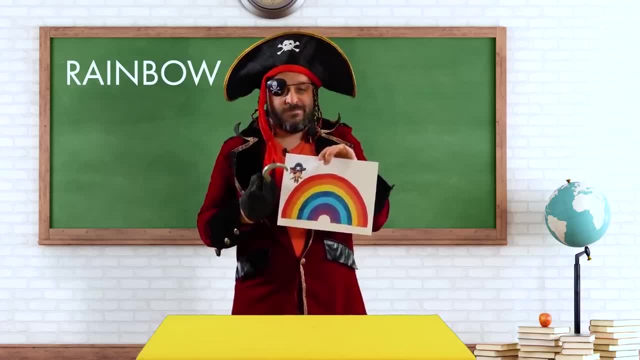 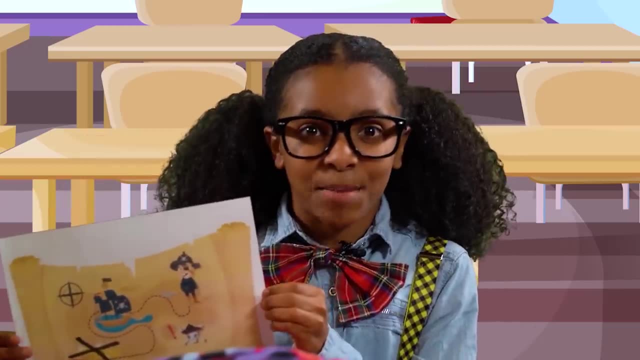 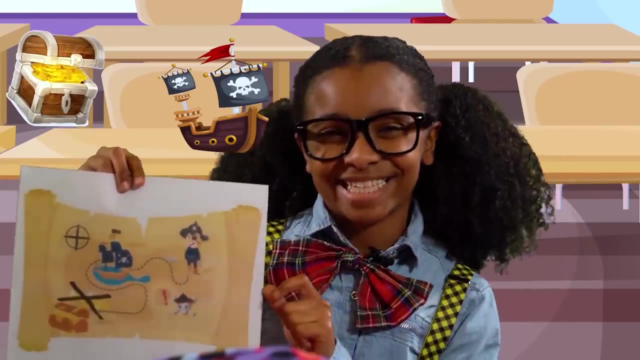 Not bad, Ellie Sparkles. Not bad. If you think that's good. look at what I have. I made it. It's a pirate treasure map. This is Pirate Island. That's a pirate ship, and the X marks where the treasure is hidden. 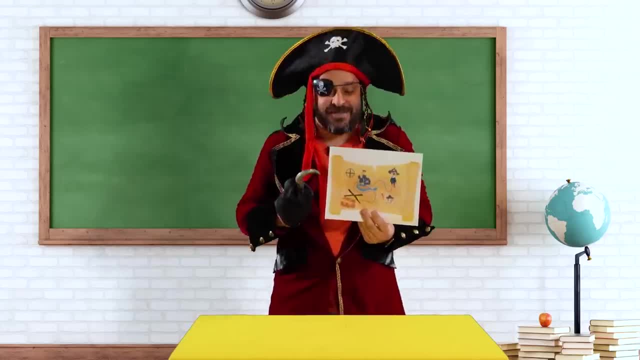 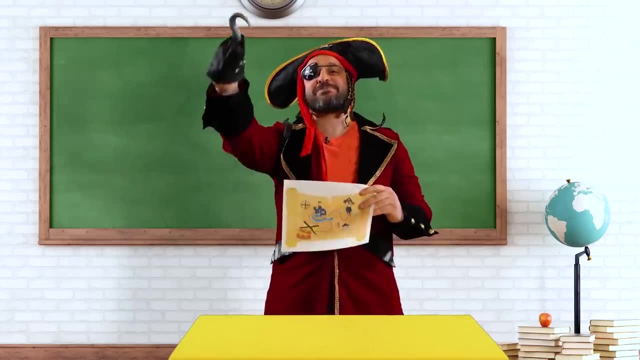 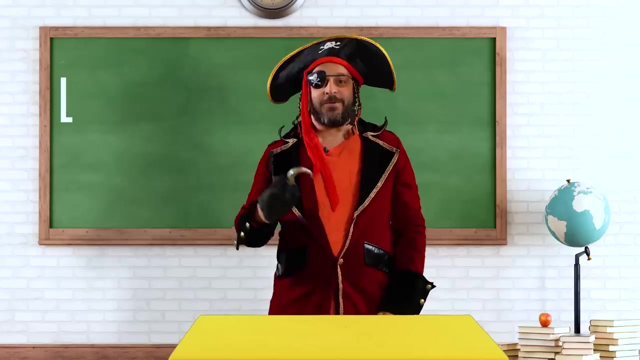 Oh, a pirate treasure map. I love it. Cool. Now I can finally find the treasure I've been looking for this whole time. I'll be the richest pirate in school. Oh, A plus for you, Alex, OK, OK, time for the first pirate lesson. 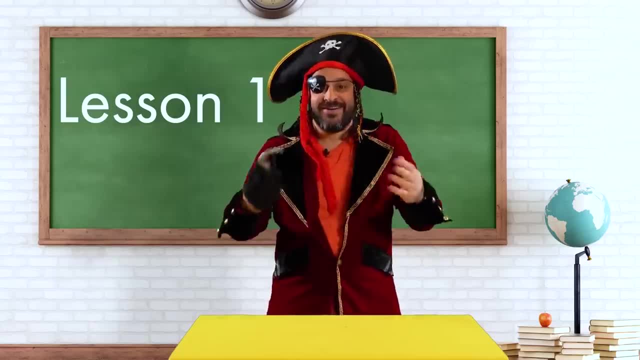 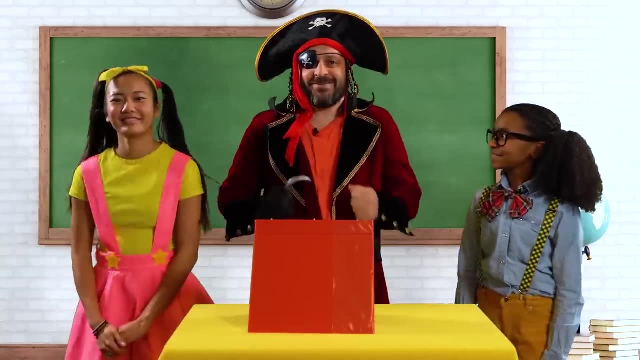 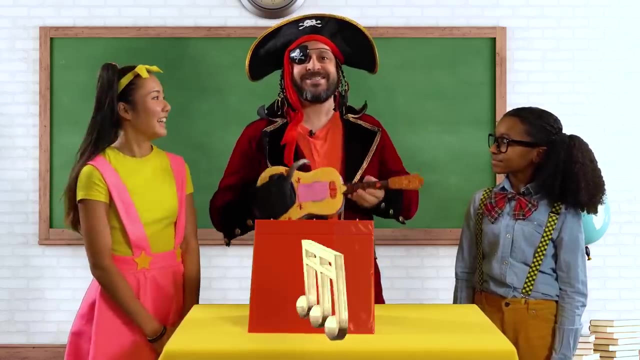 For this one. I need you both up at my desk. Come on, come on. Oh, I've been studying all week for this class and I can't wait to show you what's next. It's music class- Yes, my favorite. 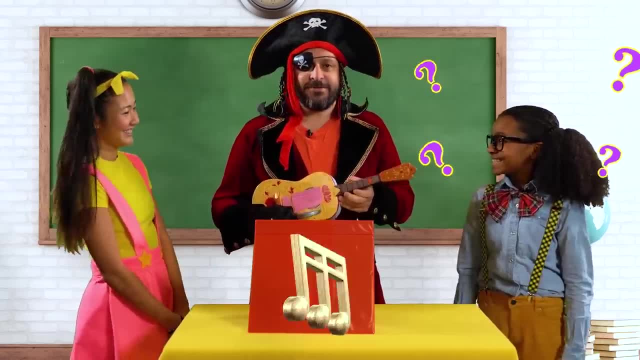 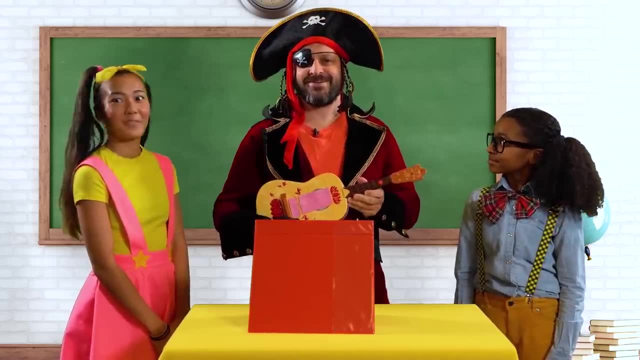 I'm the best singer in school. What song are we singing today? Well, I've got me pirate guitar, I've got me pirate music book And today we're gonna sing a pirate song. It's about all kinds of piratey things. 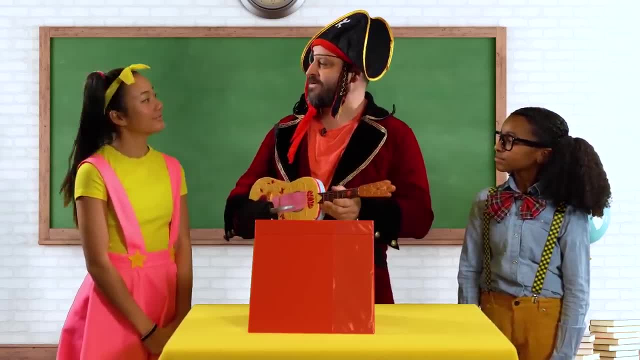 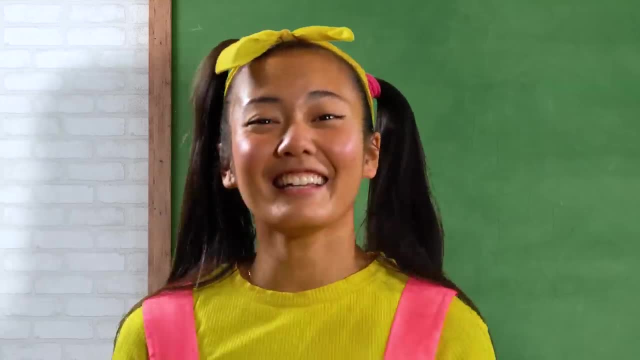 And here's what I want you to do. I'm going to start singing the song And when I stop, you guys can finish the sentence. What do you say about that? Sounds good to me. This is me pirate song. Everybody sing along. 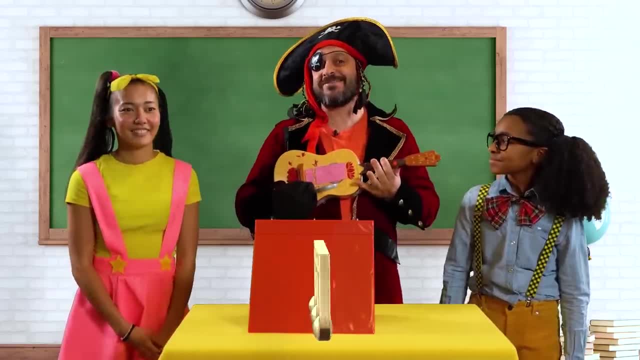 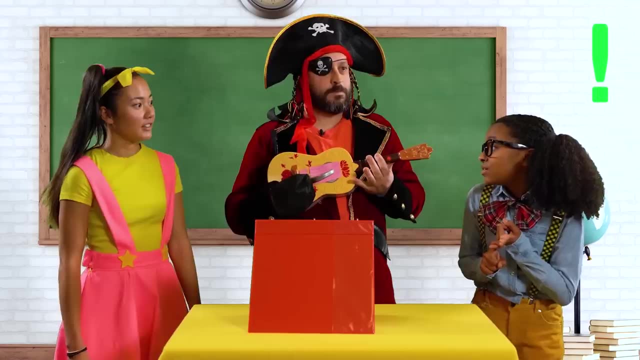 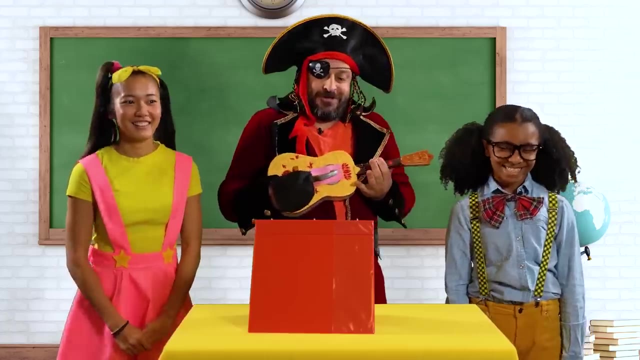 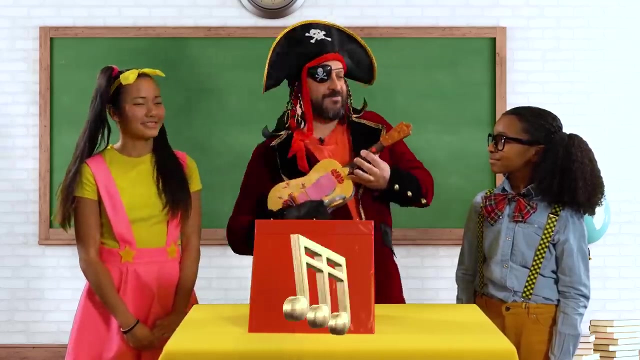 Singing for you is my pleasure. It's almost better than pirate Treasure. I was going to say, say that, but I was also going to say a pirate's parrot or a pirate hat or pirate ship. Oh, great job, Alex. you've been studying Well. it's time for the next song. Oh, I have me bird, I have me ship. 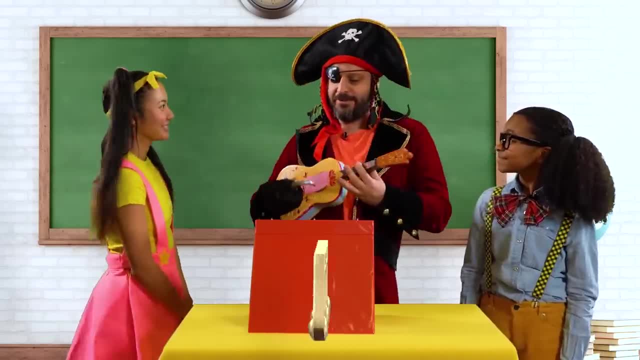 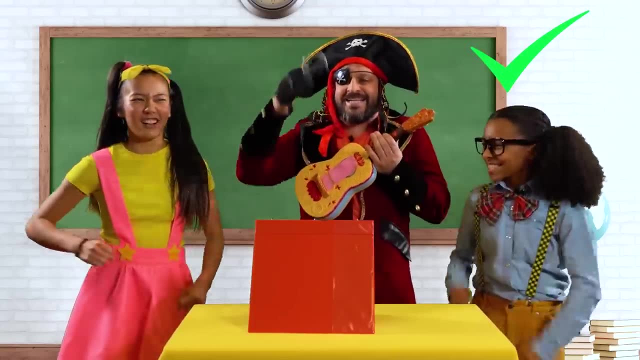 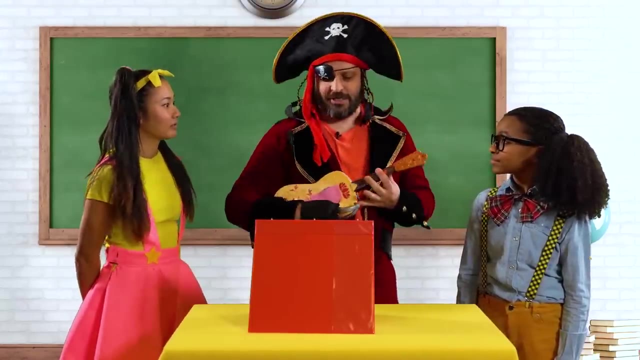 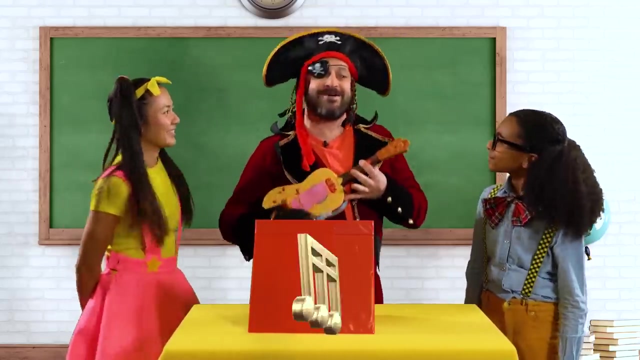 come with me and take a trip. Pirates are daring, pirates are bold and if we're lucky, we'll find them. Oh, I know I know gold. Oh right again, Alex. And the next song, this is the last one, pay attention. yo ho, yo ho, it's fun to be a pirate. yo ho, yo ho. a pirate's life for me. swab the deck, swab the deck. 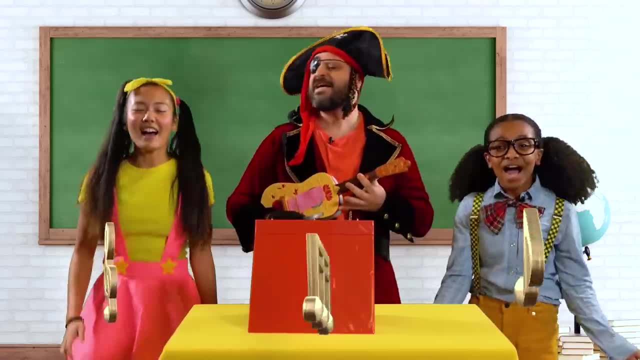 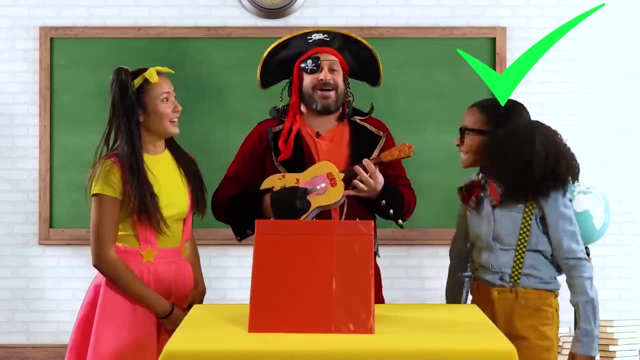 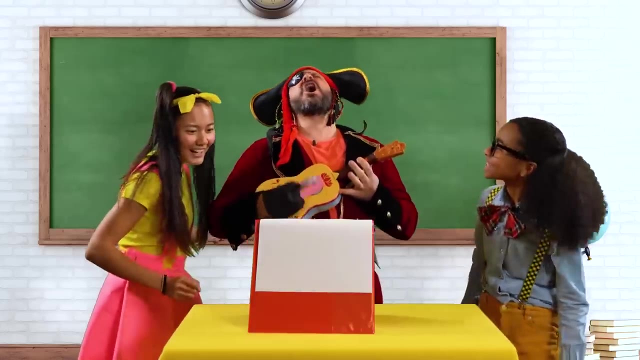 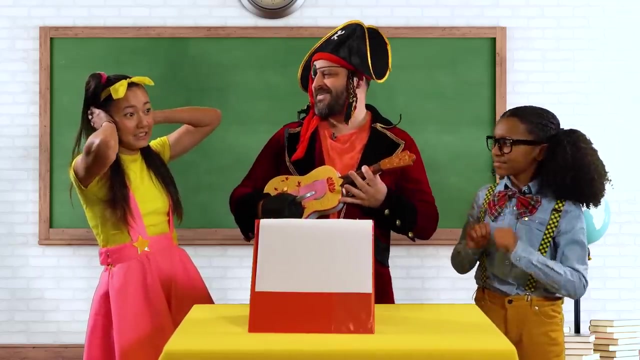 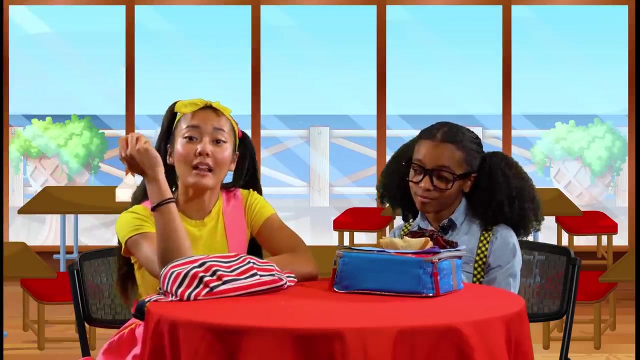 get the map. get the map, peephole, peephole, and give it all you got, because X marks the map. Great job, Alex. Oh, you're doing great. And that's the end of the pirate song. That was good, Golden pipes. Geez, what a long day of school. Only one class left of Mr Pirate and 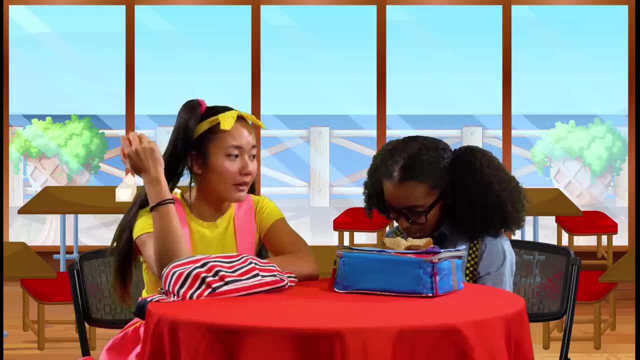 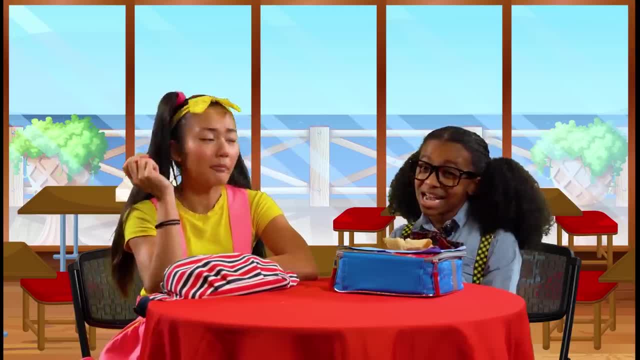 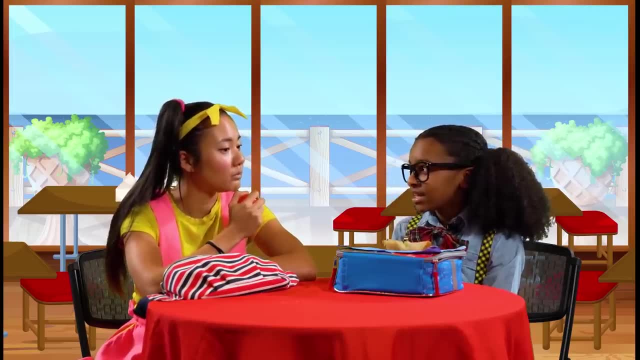 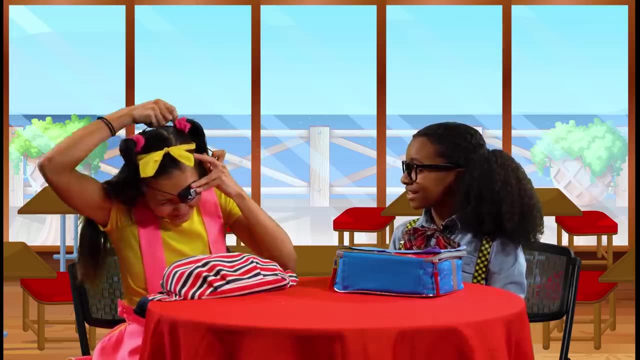 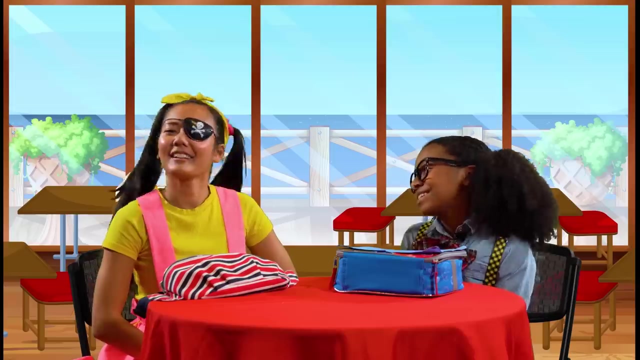 think like a pirate. Can you show me how Well? I usually don't like to share Pirate's secrets, But today's your lucky day. You just have to use your imagination, Ellie. Hey, I have an idea. Try this on. Hooray there Be, it's perfect. This should inspire you to think just like your pixel and but 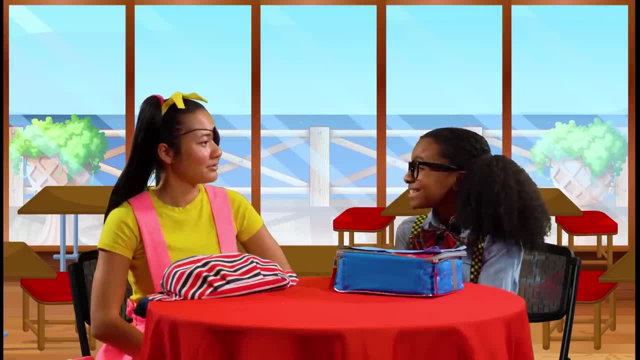 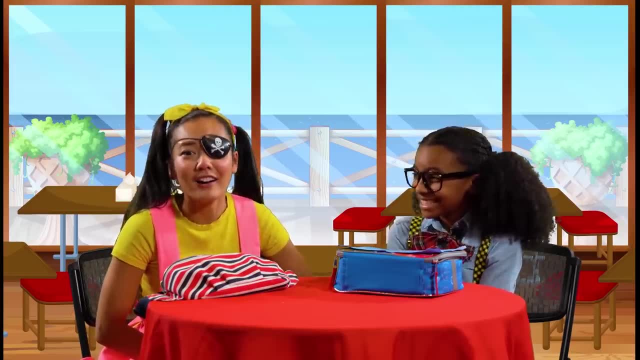 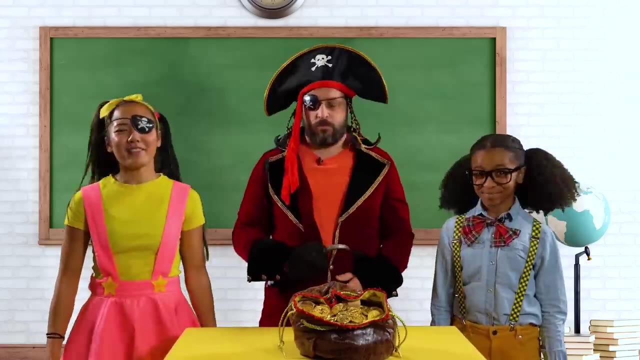 like a pirate And remember, use your imagination and just get creative. Thanks, Alex. Now where's me pirate hook? Oh see, I think it's working already. Okay, Mr Pirate, we're back from our pirate lunch. 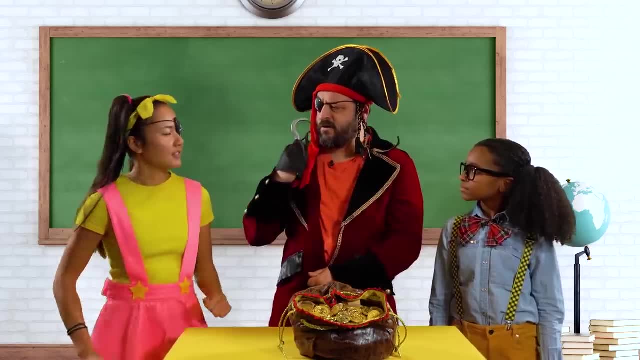 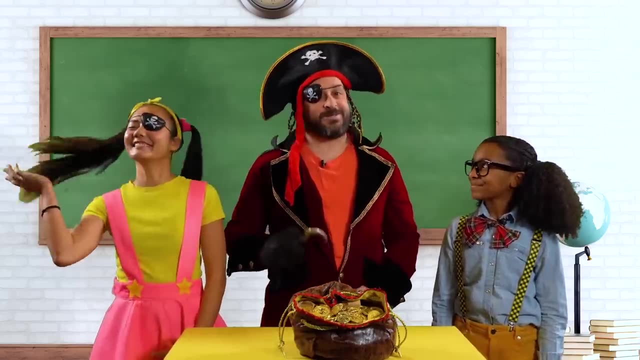 and we're ready for our final lesson. Arr Ellie, you look different. Oh, I know You got a haircut, didn't you? Well, if there's no time for haircuts now, it's time for me. final pirate quiz of the day. 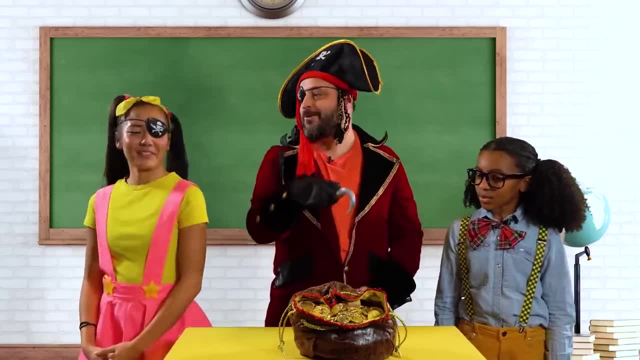 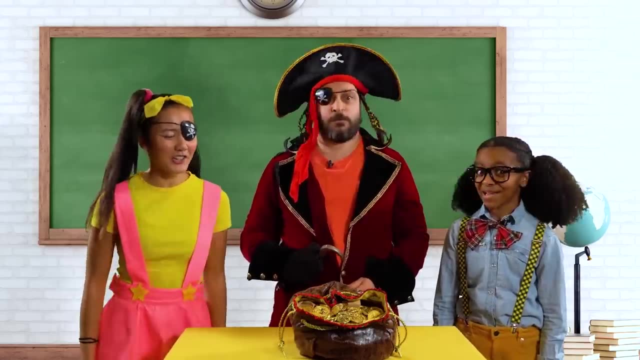 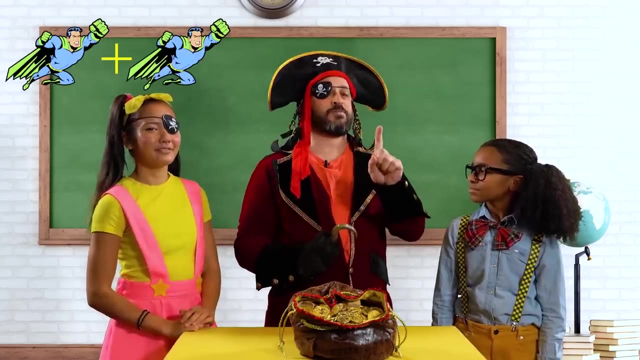 And whoever answers all my questions right gets me pirate gold. Well, no, no, not all of it, Maybe just this one. right here I'm gonna take all your pirate treasure. Arr Question number one: One superhero plus one superhero equals. 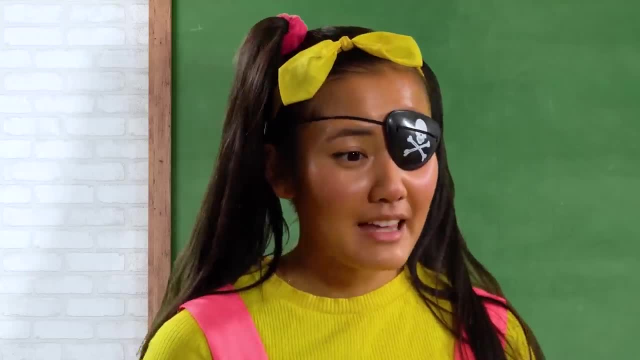 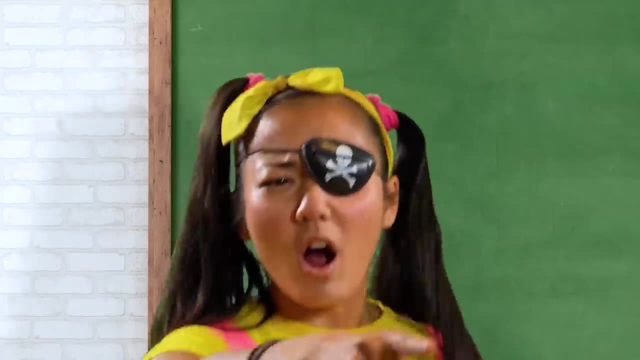 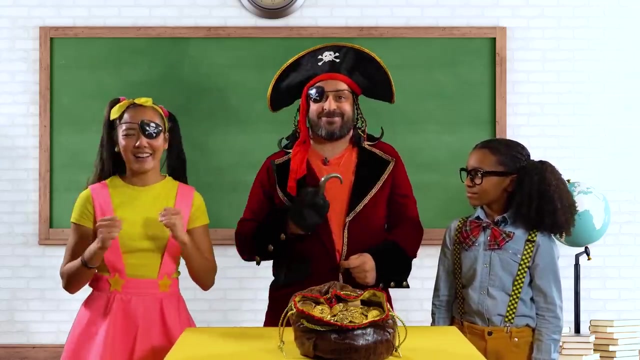 You got this, Ellie. Um, think like a pirate. One superhero, and one superhero is: Walk the plank. Shiver me timbers. Ellie, you got it right. It must be that new haircut of yours. Lesson number two: spelling. 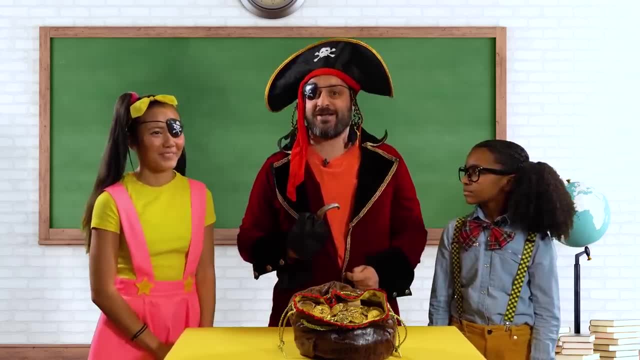 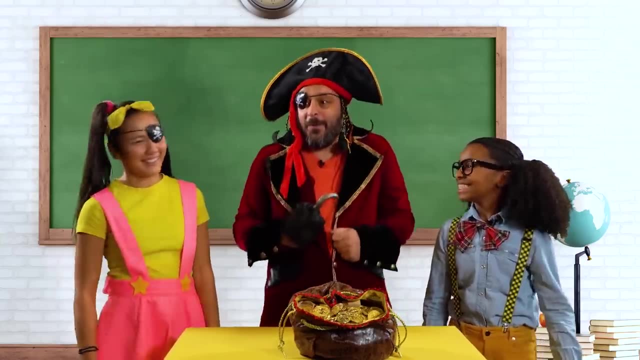 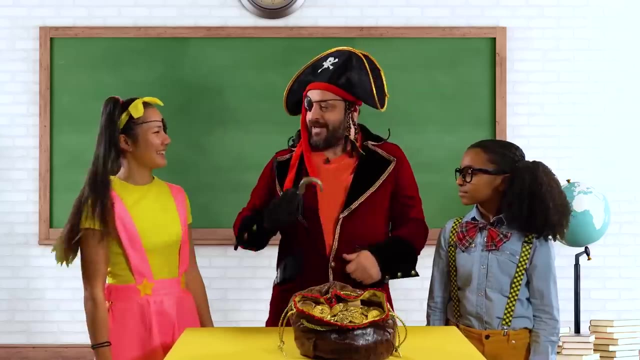 We're gonna spell me favorite word, gold. Oh easy, Gold, G-O-L-D, Gold, Gold, Ho ho ho, you got it right again, Ellie, Amazing. Yes, Time for me. last lesson of the day, ABCs. 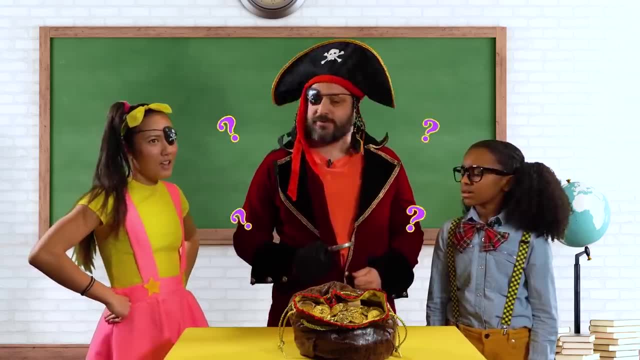 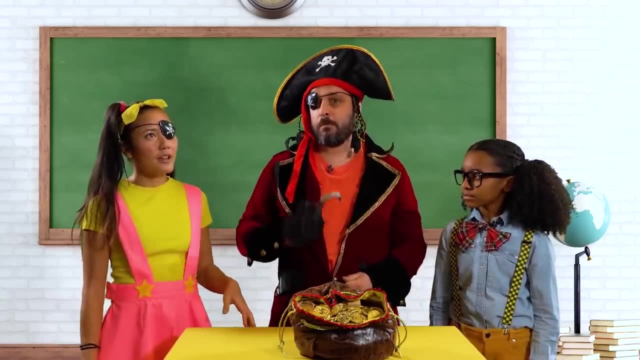 In the alphabet. what letter comes after Q, A, B, C, D, E, F, G, H, I, J, K, L, M, N, O, P, Q, Arr, Arr, Wowie, zowie. 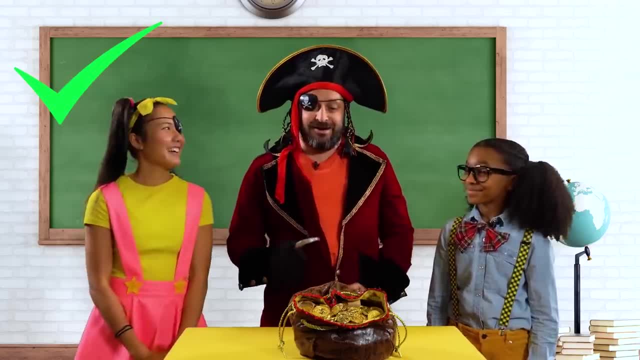 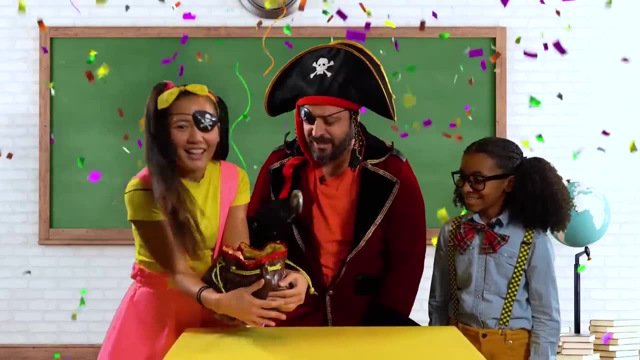 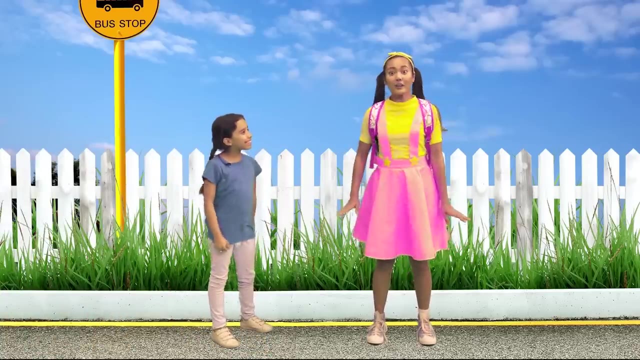 Wowie zowie, You got them all right. Now you get all me pirate gold. Oh Bye, pirate gold. I'll miss you, Especially that sparkly one right there. Hi Arwen, Are you ready for the first day of school? 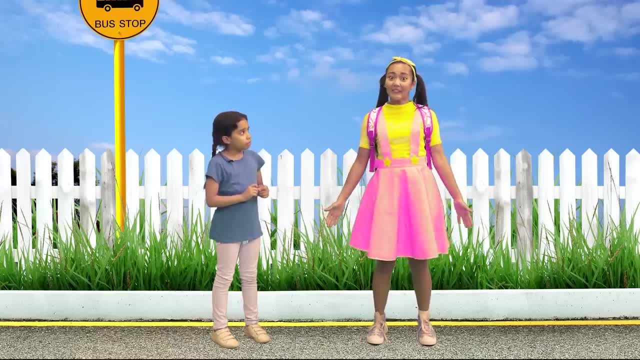 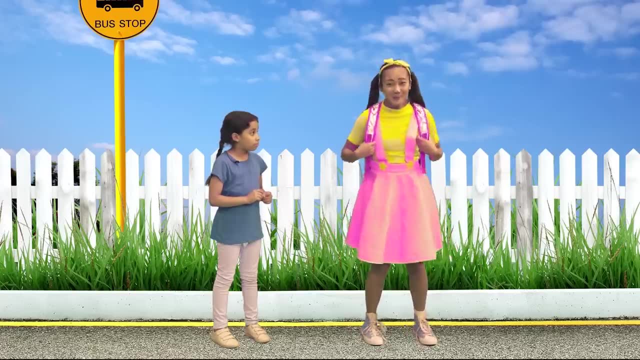 She said that she wanted us to get all new school supplies and even a new book bag, And that's exactly what I did. Look at my cool new bag. It's so heavy. I'll be the new school supplies, But, Arwen, where's your bag? 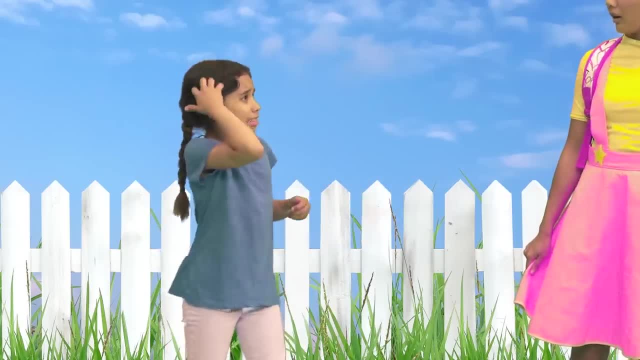 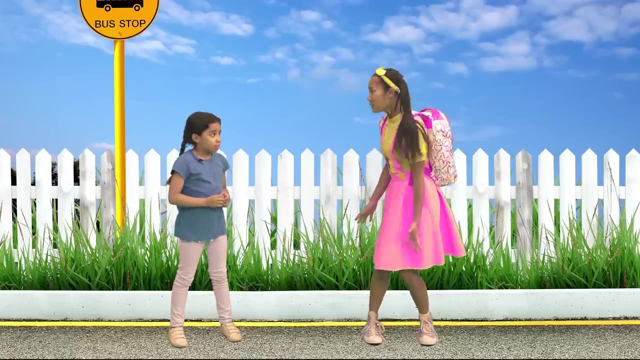 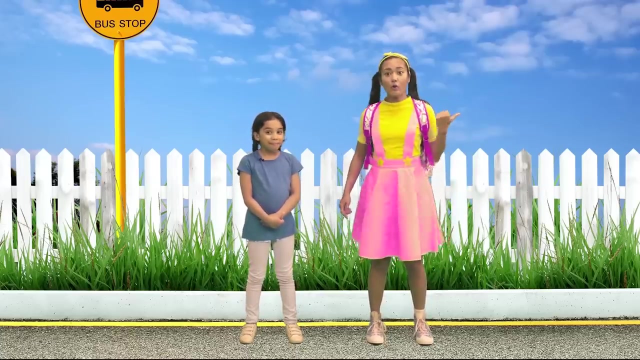 Ooh, Ooh, Huh, Hmm, Oh. no, he didn't get a new bag or school supplies. Miss Blue's not going to be so happy about that. Hmm, Wait, I have a great idea. I have an old bag and old school supplies at home. 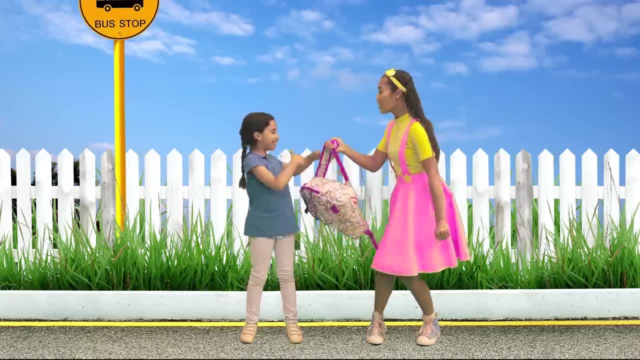 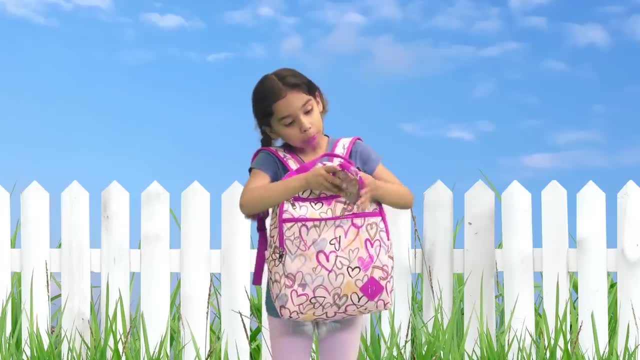 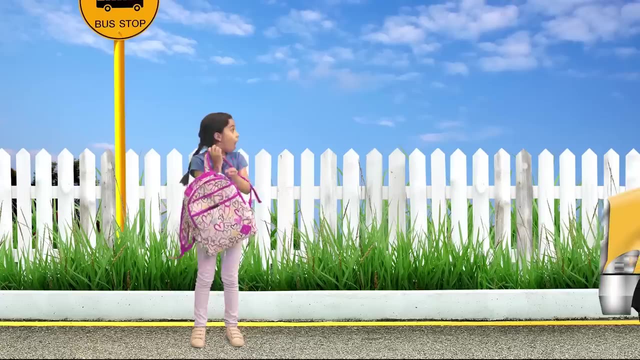 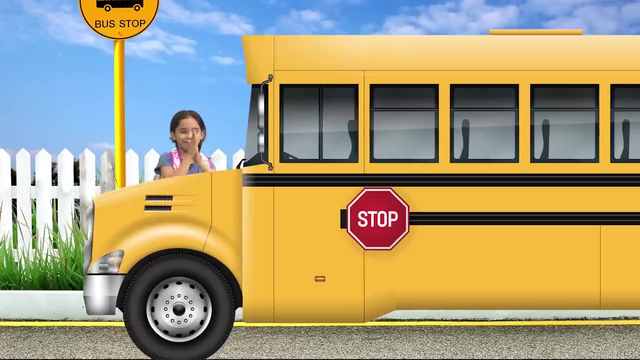 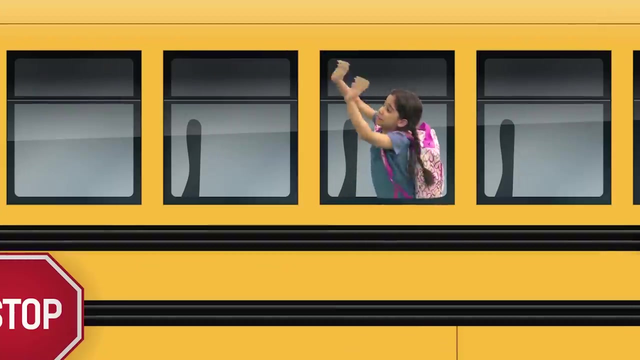 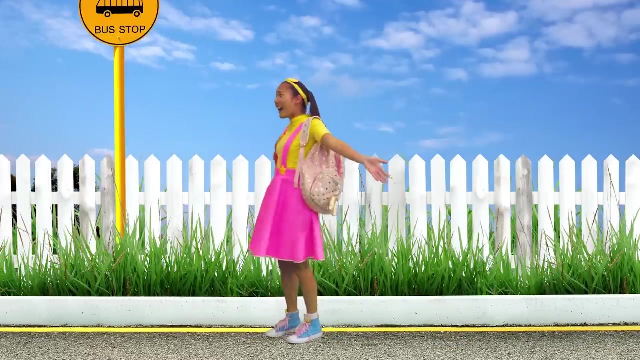 You can borrow my new bag and new school supplies today. Just make sure you hold the bus. I'll be back soon. Hmm, Hey, wait, Come back, Don't leave without me. Aw man, I thought I asked Arwen to keep the bus driver waiting. 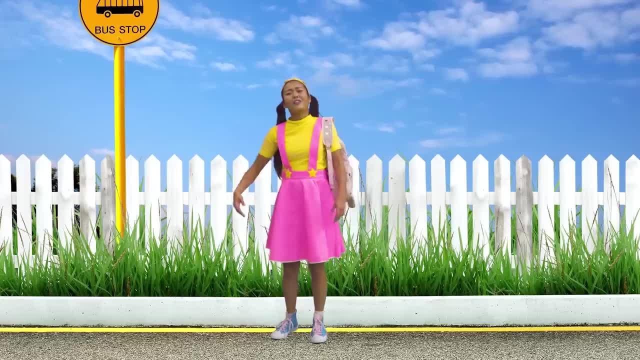 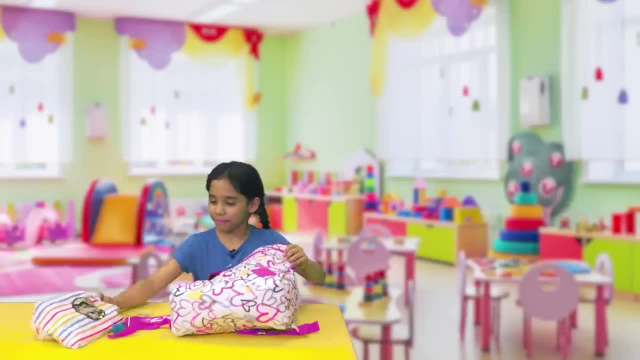 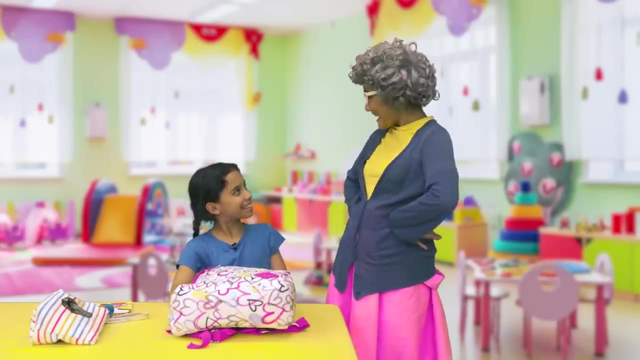 Now I'm going to be late for the first day of school. Oh, walking to school takes such a long time. Ah, it's my first new student of the day. You must be Arwen right, Woo-hoo, Woo-hoo. 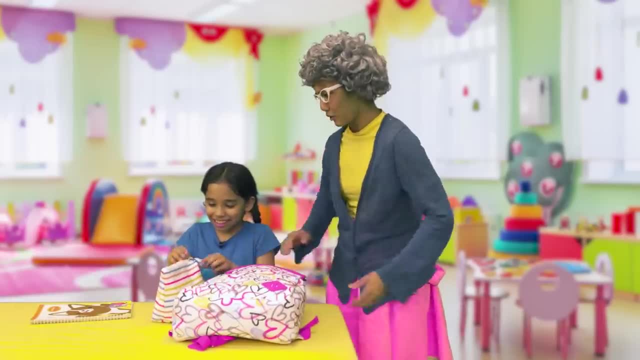 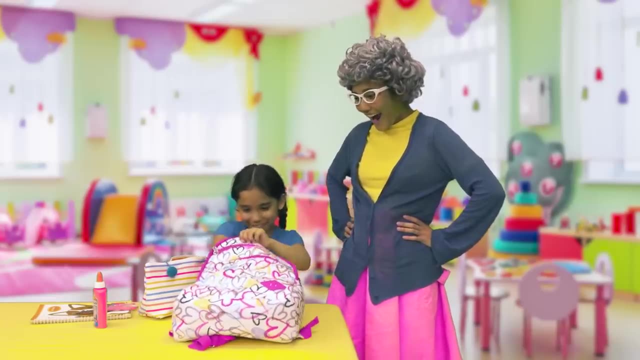 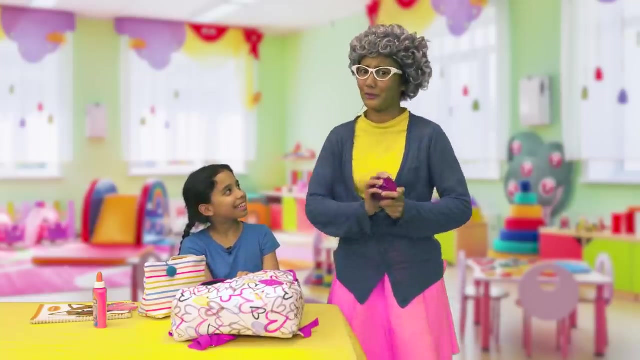 Aw, Arwen, look at your beautiful new book bag and your school supplies- Brand new. just like I asked. An apple, Just for me. How did you know? it was my favorite fruit. Arwen, you're one of my favorite students ever. 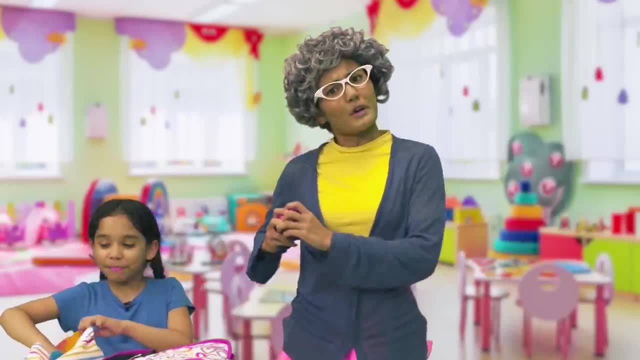 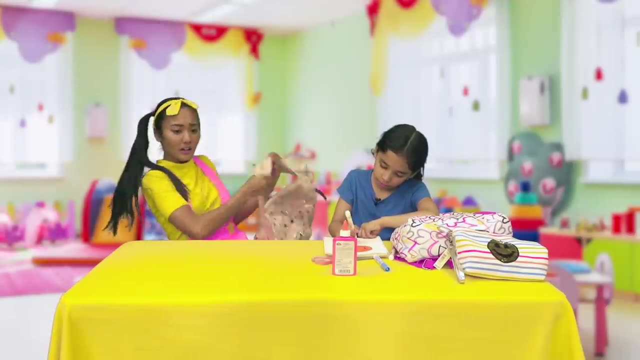 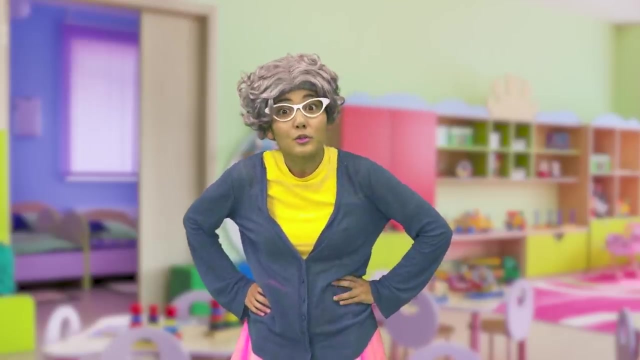 Okay, it's time to get started, But wait, We're missing one student. Where could she be? I'm here. I'm here. I made it. I see that our last student is finally here, And you must be Ellie Sparkles, aren't you? 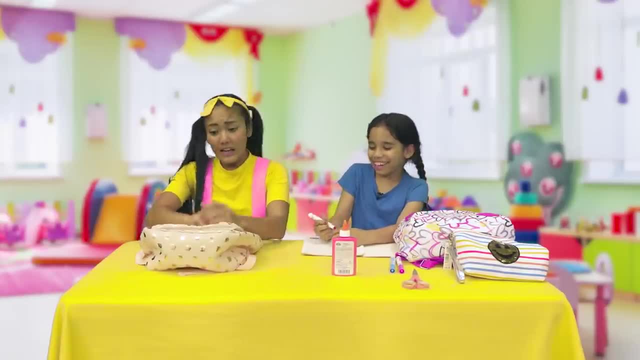 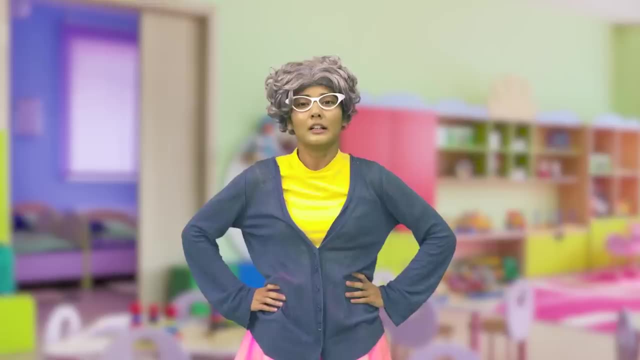 I'm so sorry I'm late. I didn't mean to be. You see, I got to the bus stop extra extra early, but then I had to run home really quickly to help a friend with her school supplies. Hmm, okay. 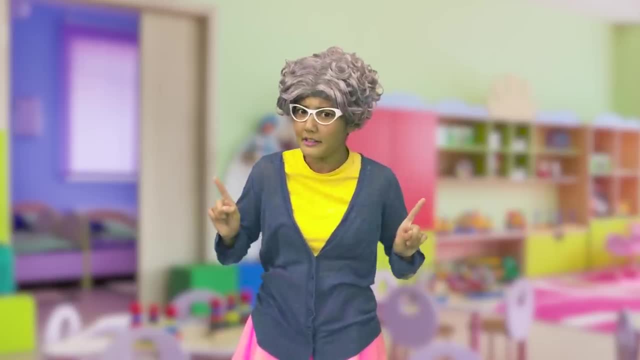 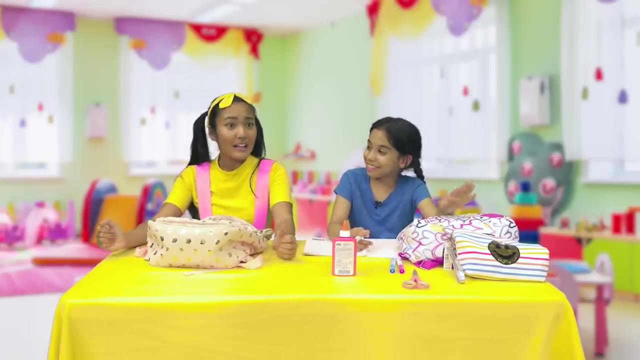 And where are your new school supplies that I told everybody to get? Oh well, I do have all brand new supplies and even a brand new book bag, but that will have to wait until tomorrow. Oh, I also got you one of your favorite treats, Ms Blue. 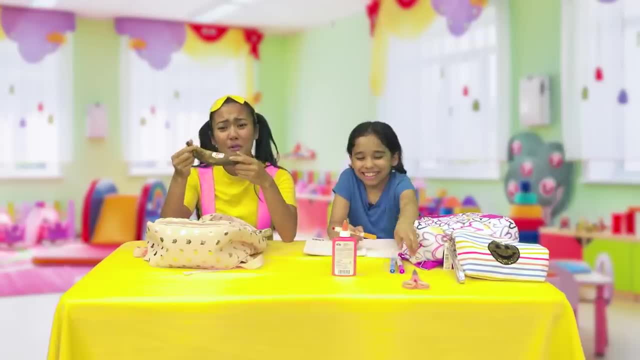 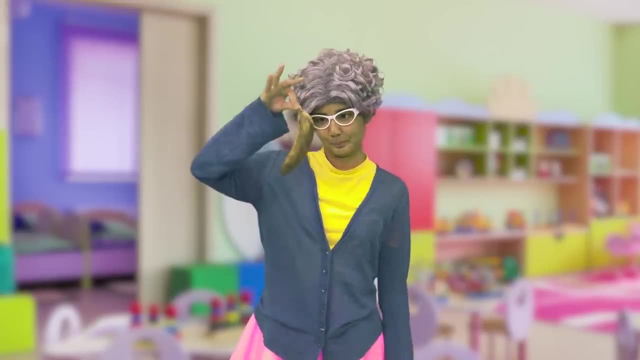 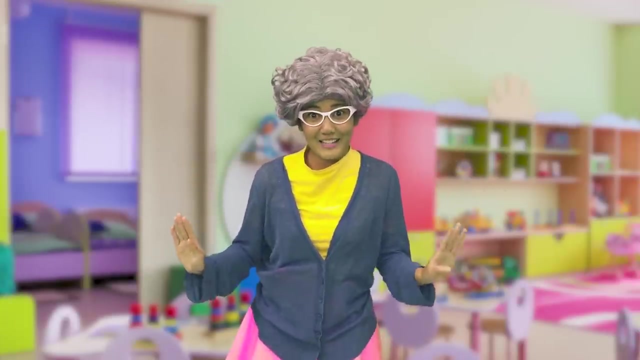 Huh, Oh no, This banana was from my book bag from last year. It's so old. Sorry, Ms Blue. Okay, students, time for class. Draw me something for your art assignment, something that you did over the summer. 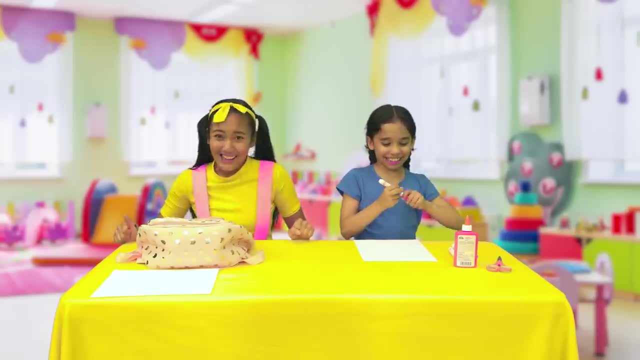 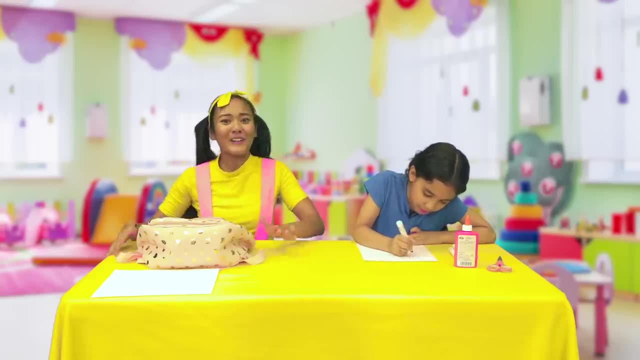 Ready, Let's go. Oh yes, Art is my favorite and best subject. Ms Blue is finally going to see I'm a good student after all. Okay, let's see what supplies are in my old bag. Oh no, 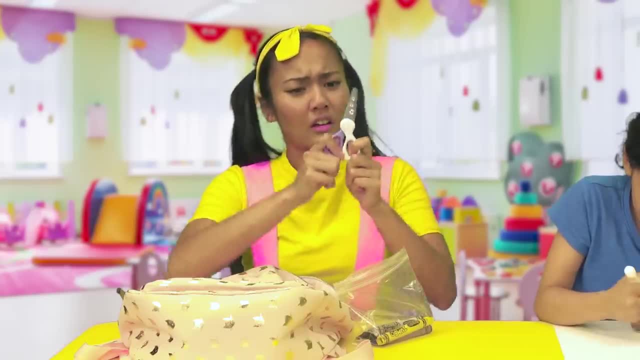 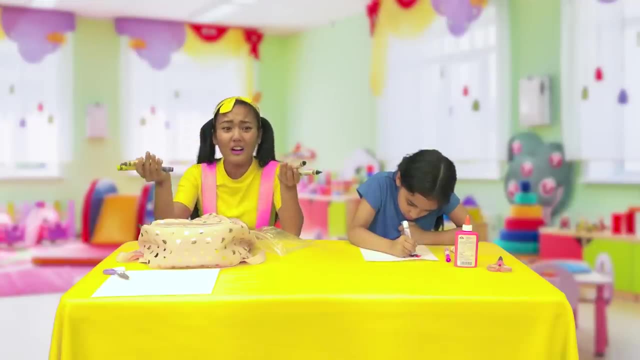 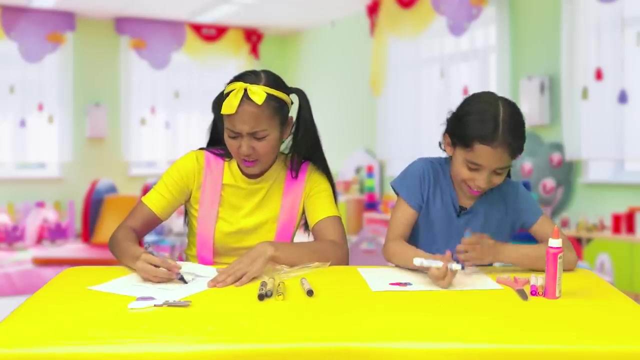 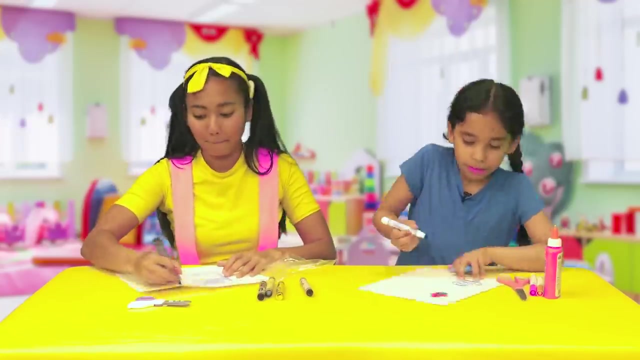 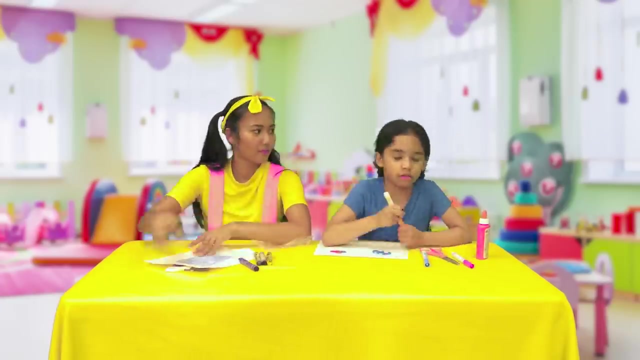 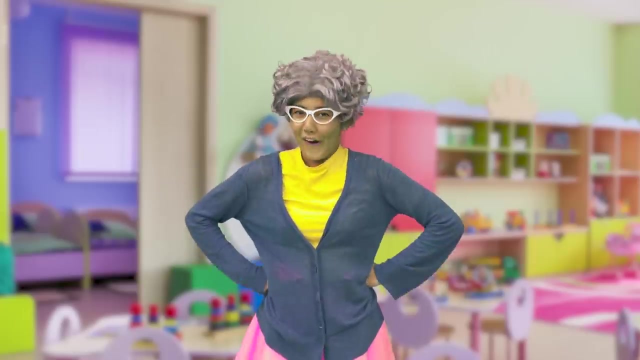 A glue bottle that's empty, Scissors that don't even work And a bunch of old crayons. Oh no, This is going to be hard. Okay, students, put down your school supplies, Since Arwen has been such a good student so far. 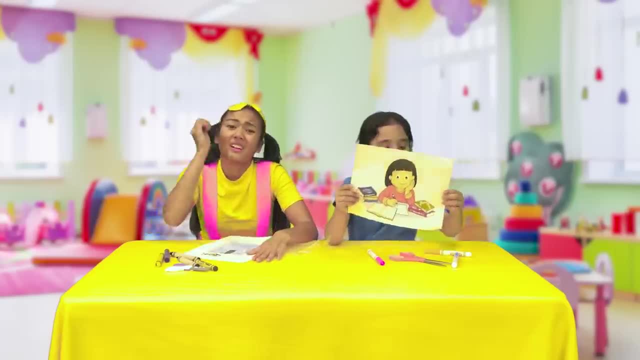 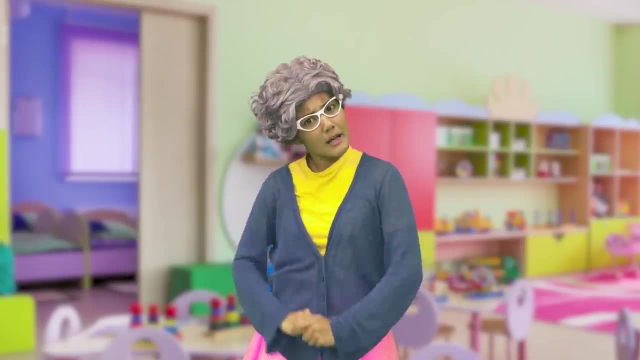 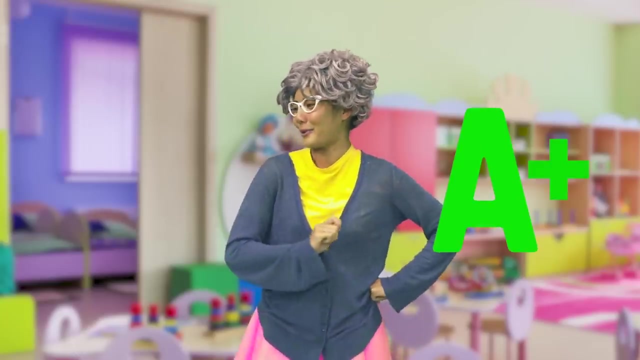 she can show us her art project first. Oh, Arwen, you spent your entire summer studying and doing homework. Oh, I can tell that you love school. so much A plus for you, Arwen. Okay, Ellie Sparkles, it's your turn. 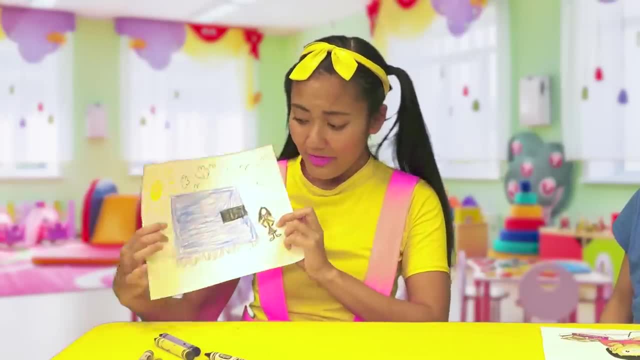 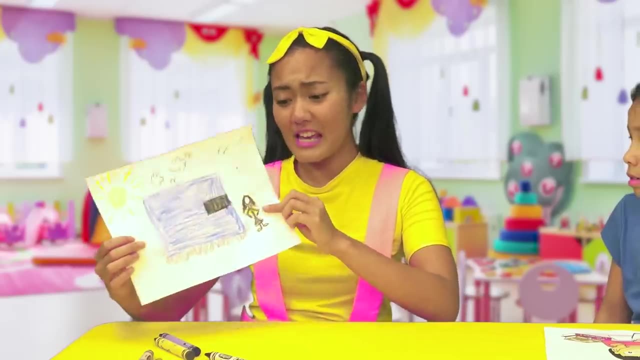 Here it is, Ms Blue. It's me at the swimming pool. That's what I did a lot during the summer. I'm so excited. I'm sorry it's not as good as I want it to be. I didn't have many colors of crayons from my old school supplies. 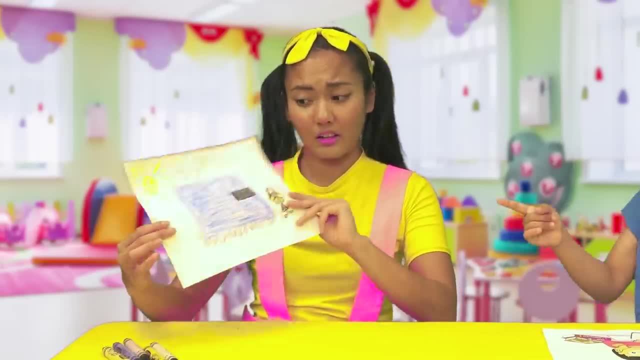 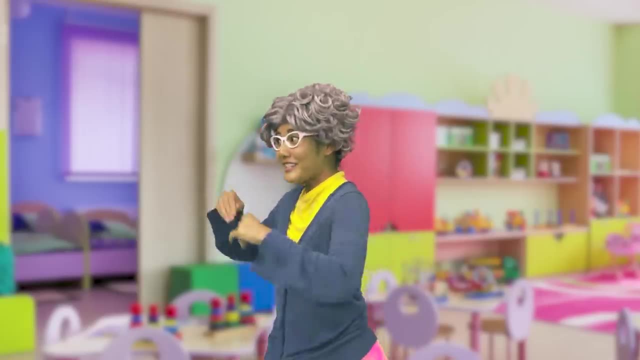 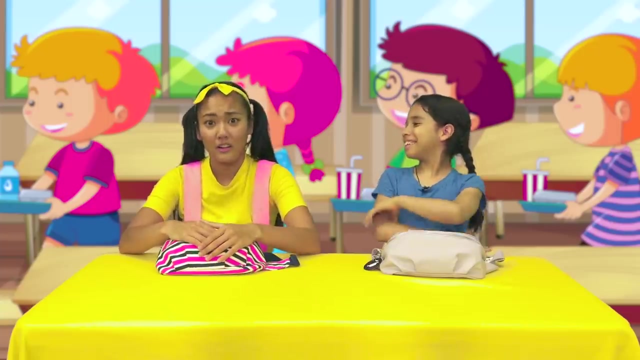 But next time I'll definitely make a better picture. Okay, class, it's time for lunchtime. Go to the cafeteria. Oh man, I've been having a really long first day of school. so far, Arwen, Ms Blue seems to really like you a lot. 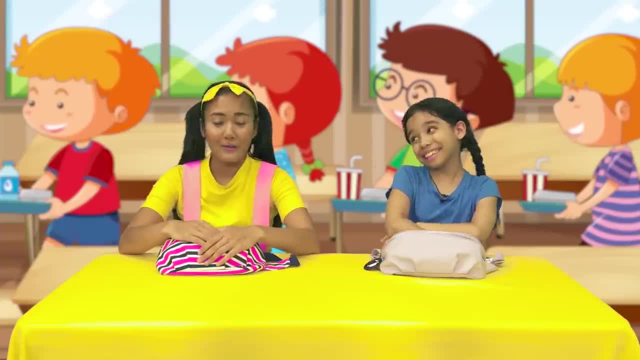 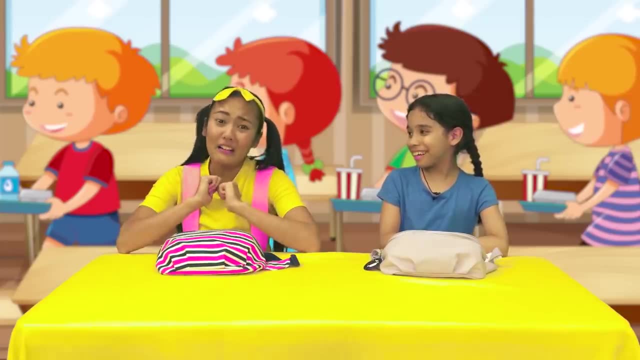 First you were early to class and then you had new school supplies and you even had a really cool art project. But I don't think Ms Blue likes me a lot. I was late to class, I had old school supplies and my art project was so bad. 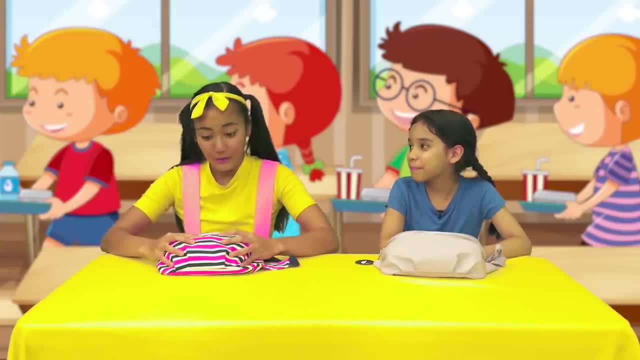 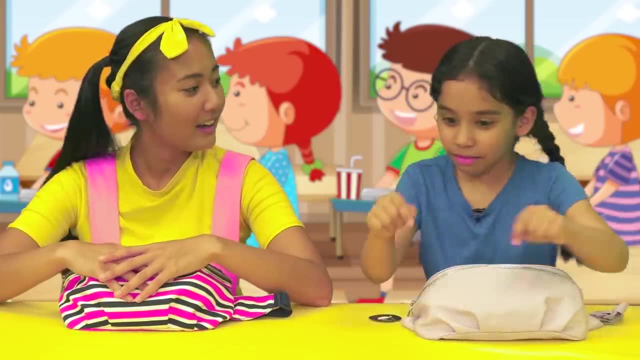 But at least I have lunchtime to look forward to. Oh, this will definitely make me feel a lot better, because my new school supplies are really cool And my lunch is really really good and yummy. Wait, you want to play lunchtime swap? 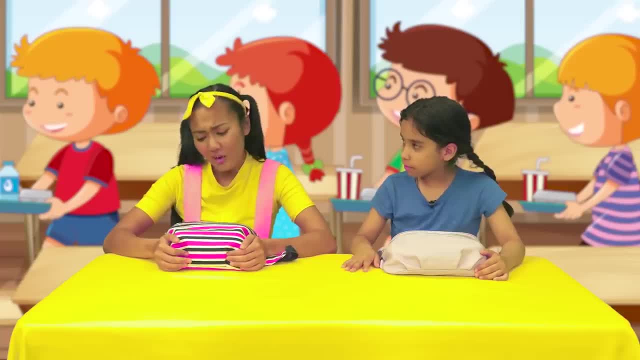 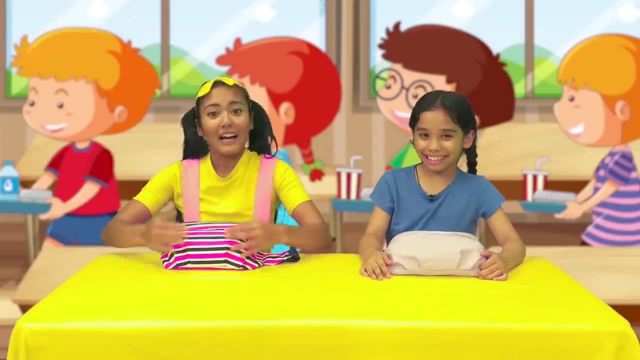 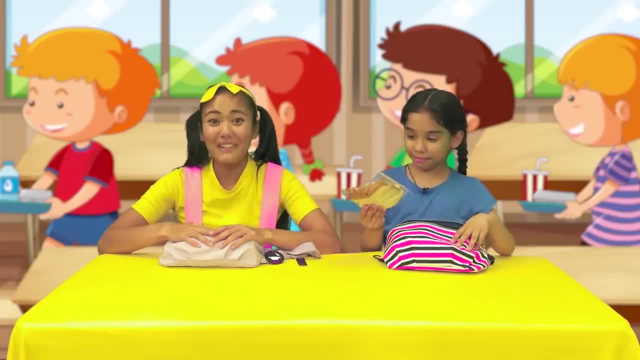 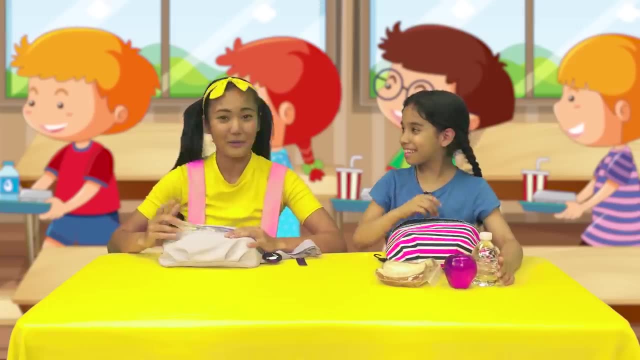 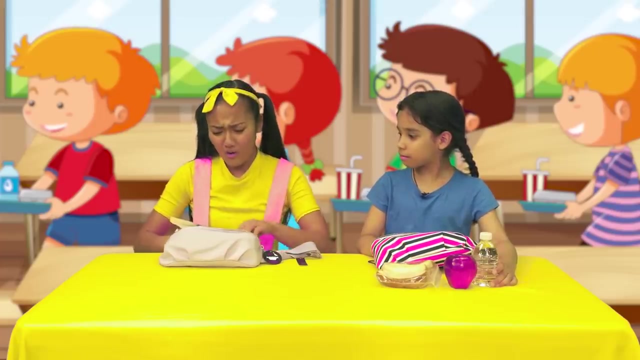 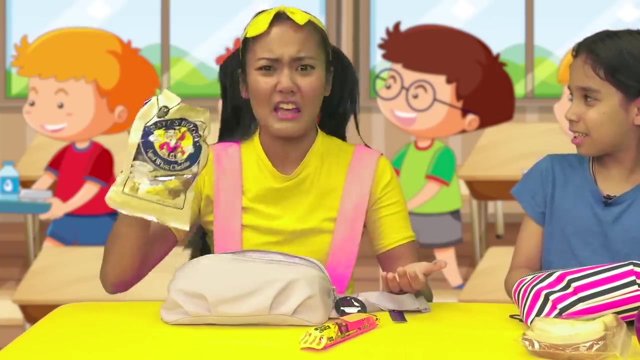 Oh no, You got a peanut butter and jelly sandwich, a bottle of water and an apple. See, I told you my lunch is really, really healthy. Okay, let's see what I got. Oh no, I got a candy bar, a half-open bag of chips and a big bottle of soda. 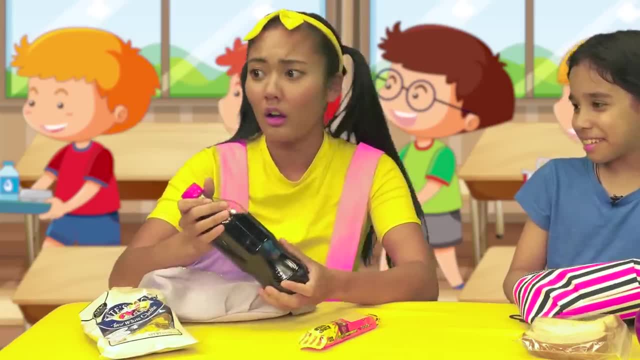 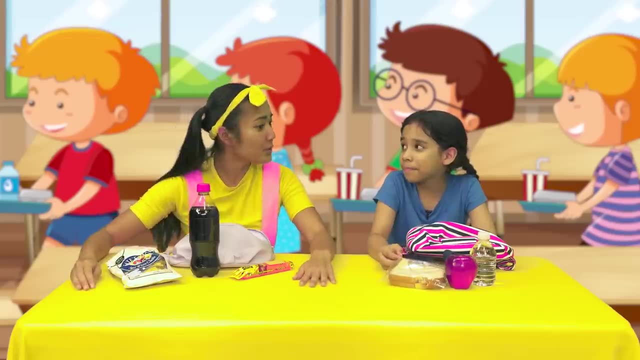 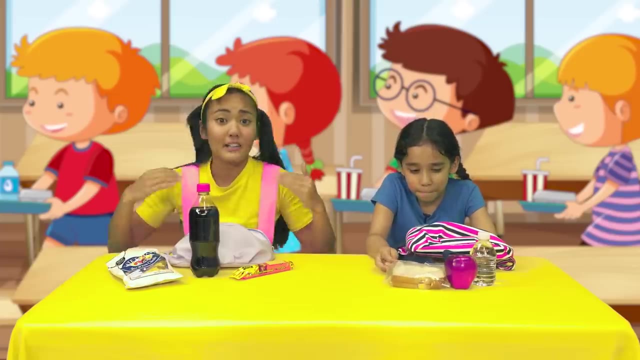 Oh, no, Oh, this isn't good at all. Huh, Oh, no, Oh. Miss Blue saw what my lunch was. Oh, this is the worst first day of school ever. I planned all summer to have the best school supplies and the best lunch for my first day. 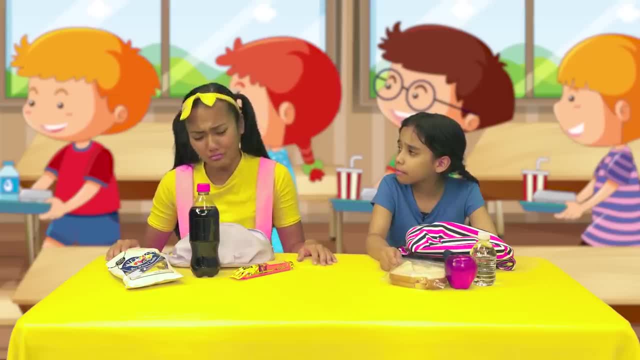 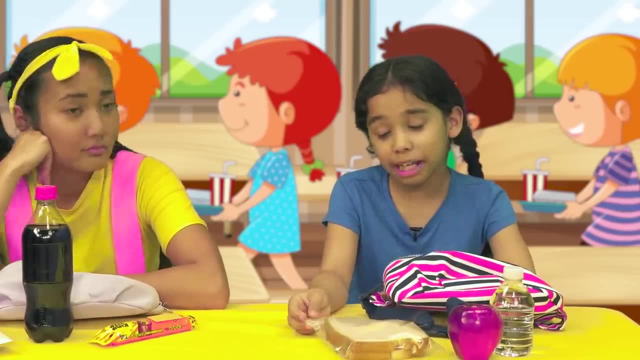 And now none of that came true. What am I going to do now? Huh, Hey, Ellie, I'm sorry for making you have a bad day in school today. Why don't you have the half of this peanut butter jelly sandwich- and I have the half of it too. 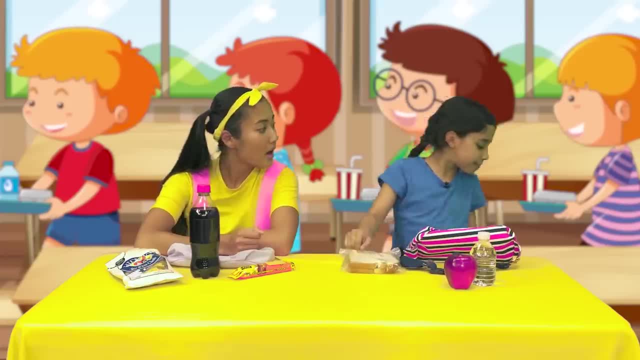 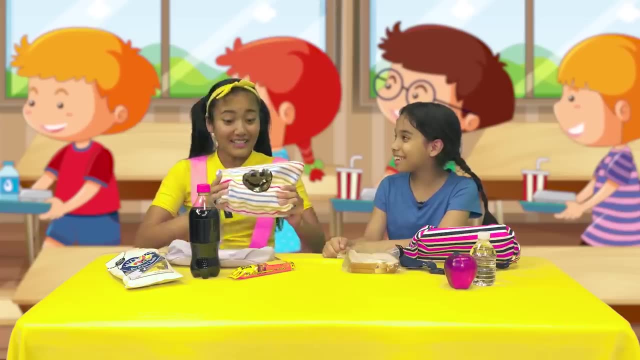 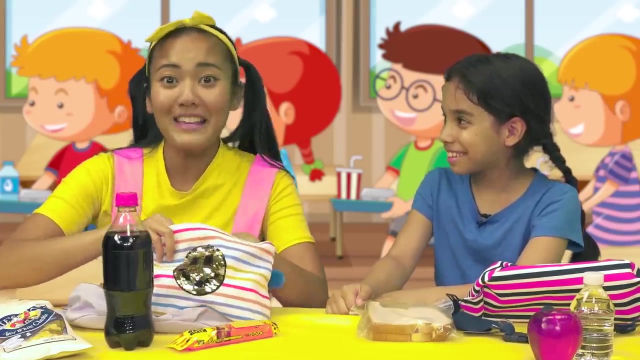 That's so nice of you, Arlen. Thank you so much. And here's your art supplies too. You can make another art project after lunch. That's such a good idea. I'll impress Miss Blue after that. Oh, this is so exciting. What about you help me out? 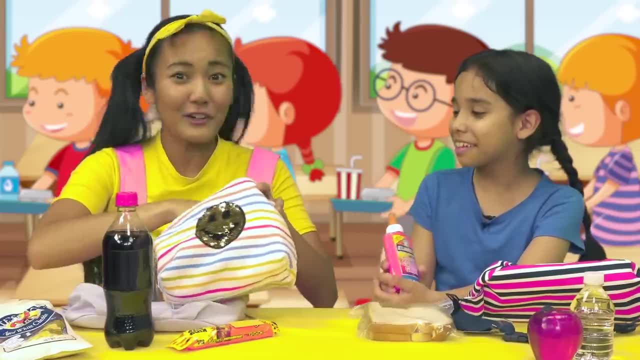 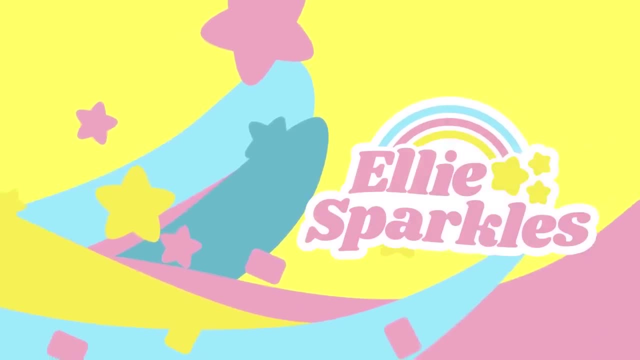 I know you're so good at gluing so you can glue. Oh, and I got these really cool markers. They actually smell like different types of fruit And oh my gosh. have you seen? Oh my gosh.